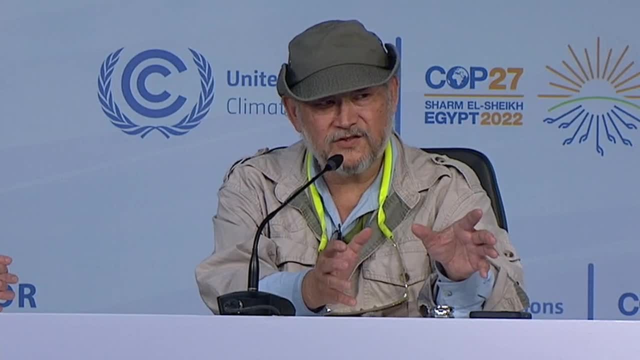 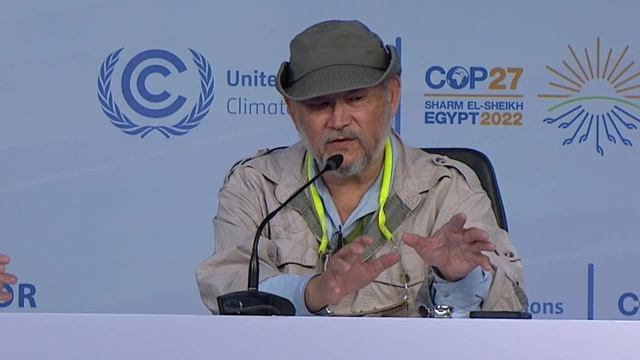 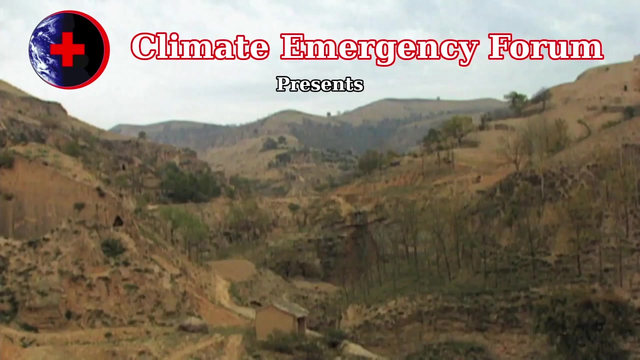 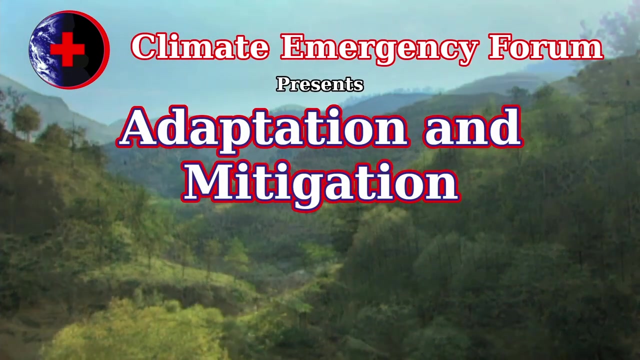 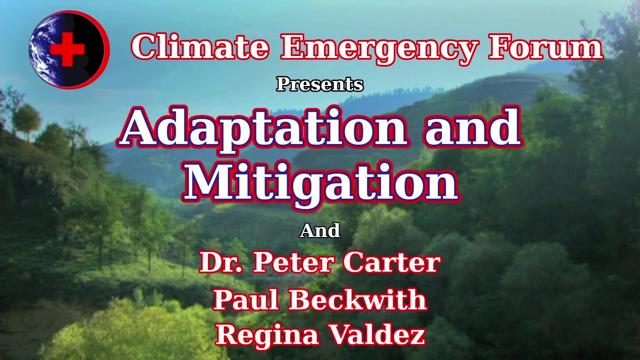 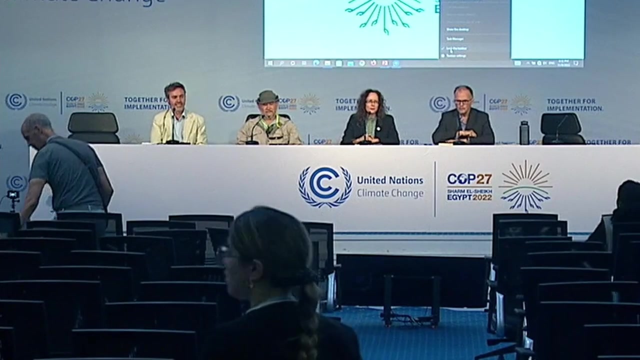 So, essentially, we learned that it's possible to rehabilitate large-scale damaged ecosystems, including ecosystems that have been damaged over very vast areas and over long historical time. Hello everyone and thank you for being here today. Sorry for the little bit of confusion. 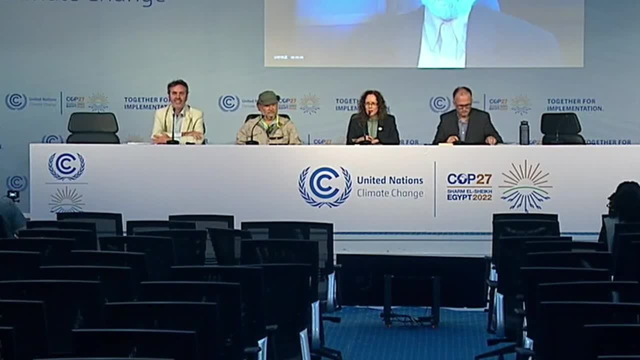 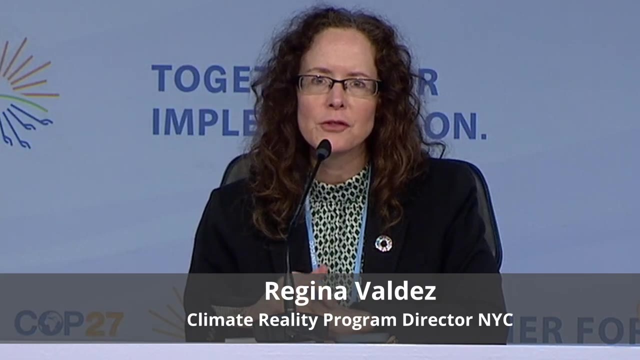 Our panel is going to be discussing a very important topic, which is mitigation and adaptation. We have a very esteemed panel. We're going to start with recorded statements from Dr Peter Carter and I will do a general introduction. I'm going to start with Dr Peter Carter. 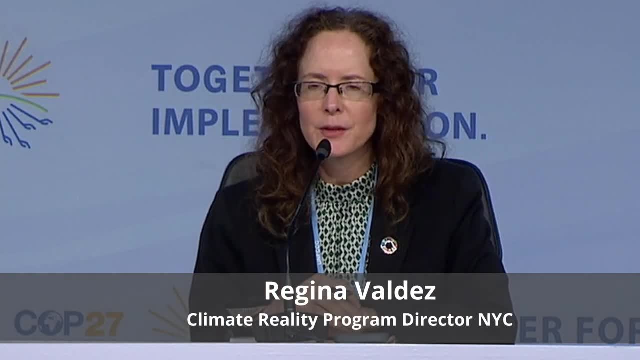 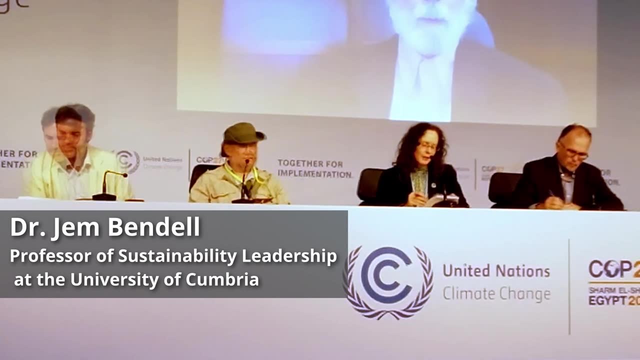 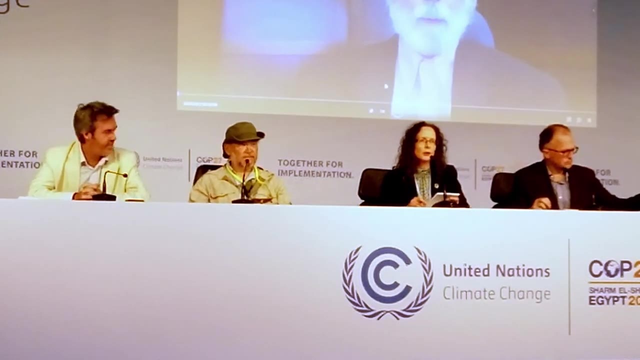 and I will do a general introduction of the people also sitting with me. To my far right is Professor Jim Bendel. He is a professor of sustainability leadership at the University of Cumbria, And to my near right is John Liu. John Liu is a journalist, filmmaker. 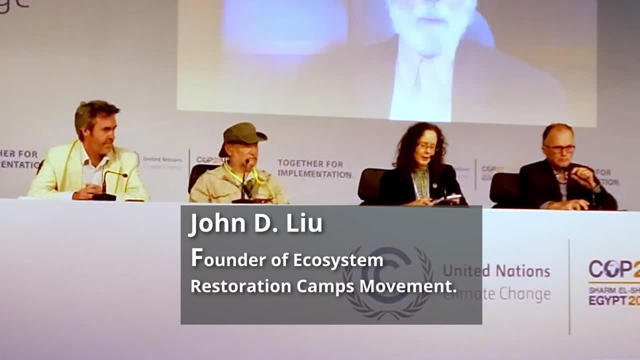 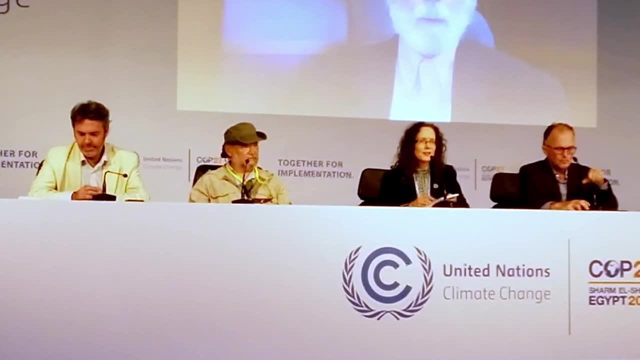 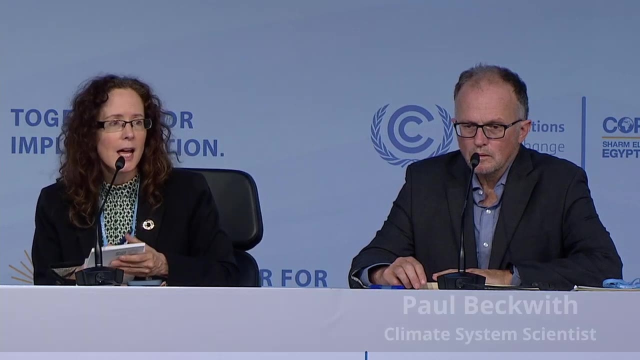 and founder of Echo Restoration Camps. There are 55 of these Echo Restoration Camps on six continents. This is a feat that he has achieved in six years: Six continents in six years. And to my left I have Paul Beckwith, who is a climate educator, and he's very well known. 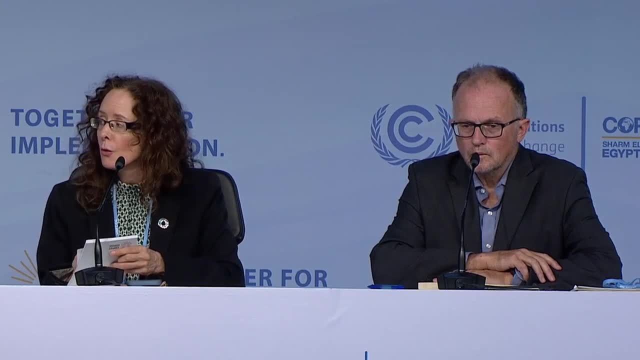 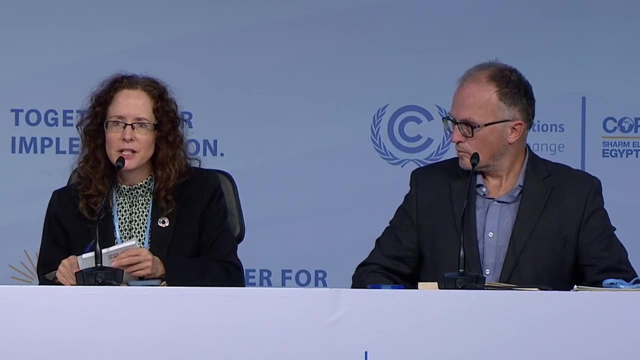 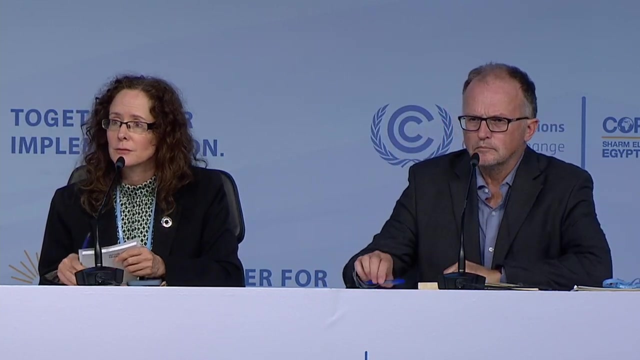 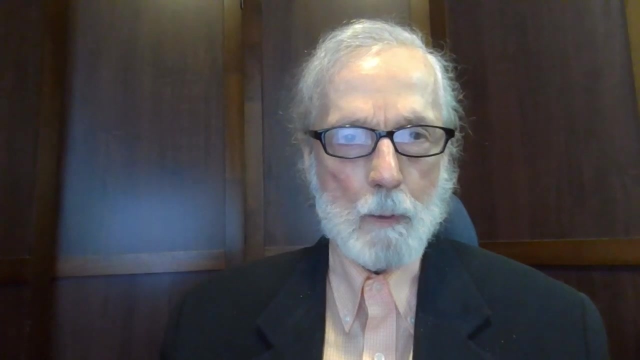 and followed on YouTube. So, without further ado, I would like to get into this discussion on the importance of adaptation and mitigation, and I would like to begin with a recorded statement from Canada, from Dr Peter Carter. Hello, the huge issue of adaptation to climate change is covered by working group. two of the 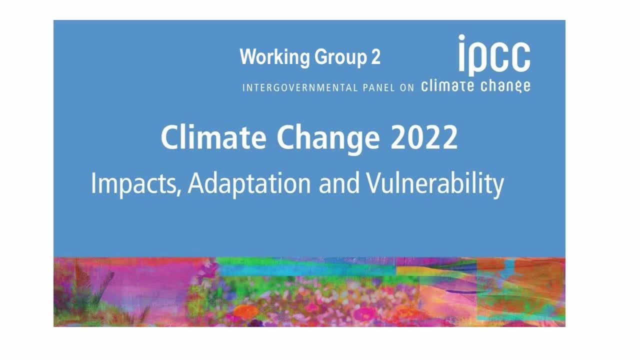 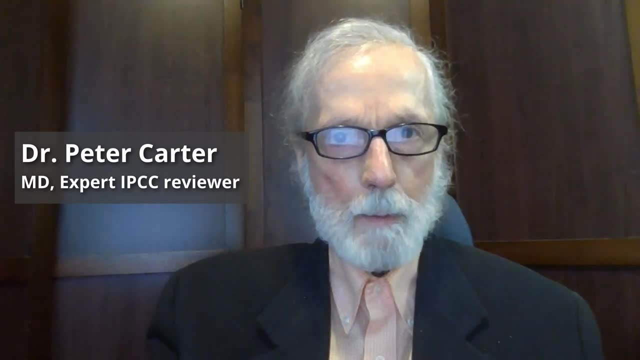 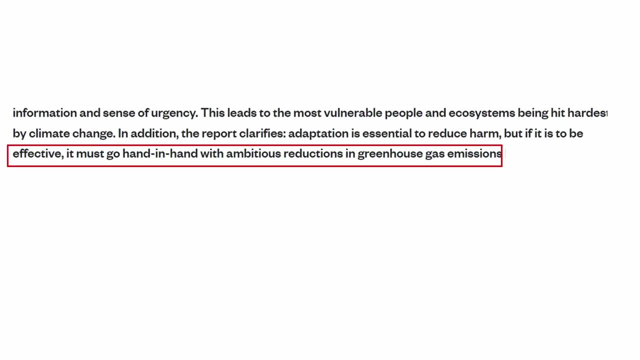 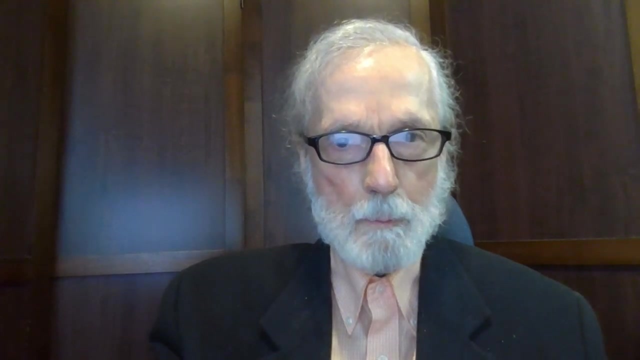 IPC Sixth Assessment. I have selected some extracts. The first one: climate change is a global threat to which all people and ecosystems are vulnerable. To be effective, adaptation must go hand-in-hand with rapid deep cuts in greenhouse gas gas emissions. There are limits to adaptation that depend largely on resilience, But as temperature 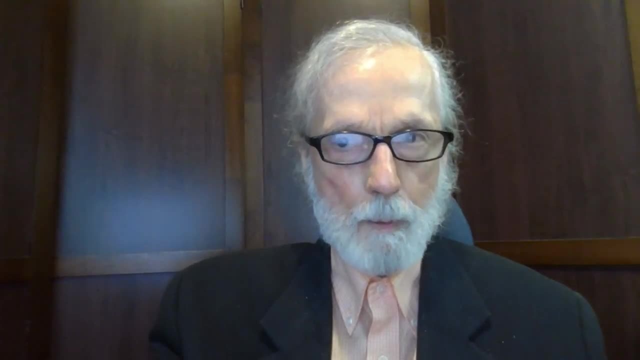 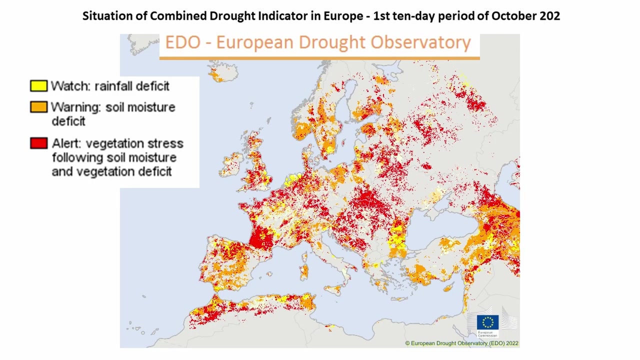 increases, resilience decreases And then we have extreme weather events. We are near those limits even in the Northern Hemisphere- The Northern Hemisphere- summer of this year, 2022, of unprecedented extremes right across the Northern Hemisphere. Today, 42% of Europe is still in drought and 60%. 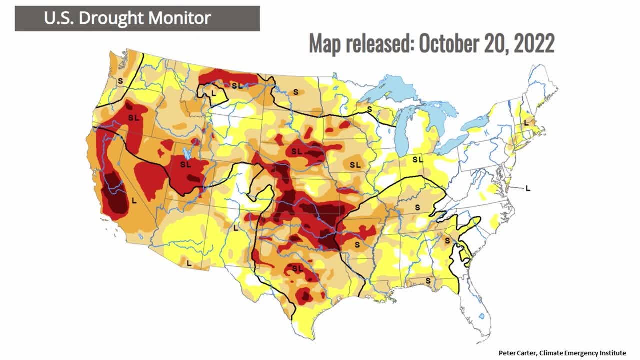 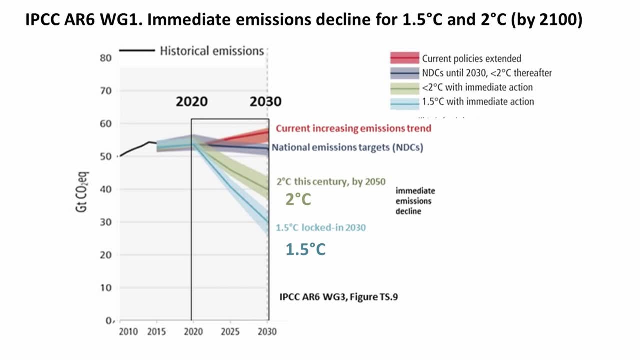 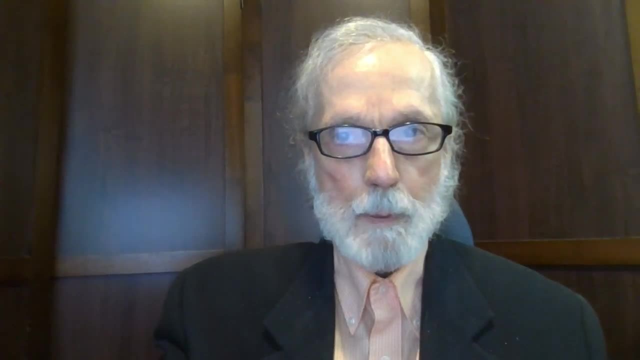 of the US is still in drought. Clearly we have no more time left. Working Group 3 says that global emissions have to decline immediately for 2C as well as 1.5C. The report finds that many species and ecosystems are currently near or beyond their adaptation limits and people that rely on them to survive. That single quote says it all: 3.5 billion people live in contexts that are highly vulnerable to climate change. Africa: Since 1961, crop productivity growth in Africa shrunk by a third due to climate change. So Africa has to be prioritized for funding and assistance for adaptation development. 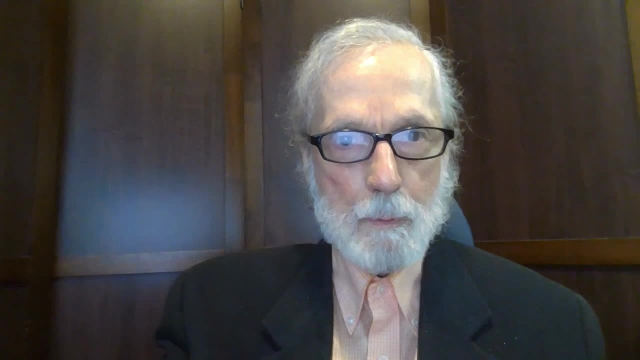 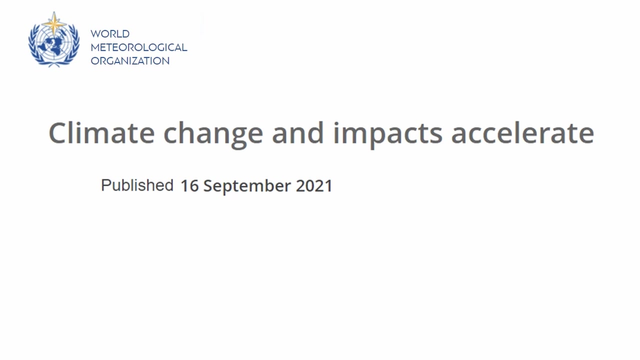 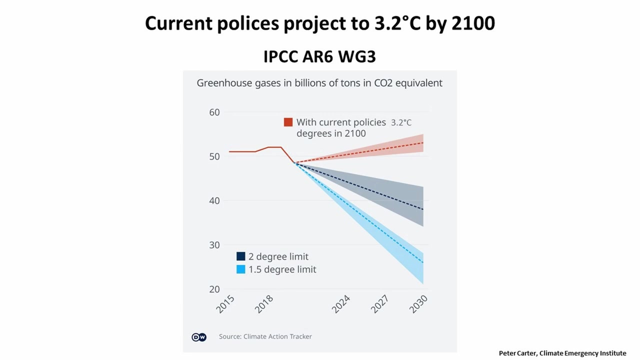 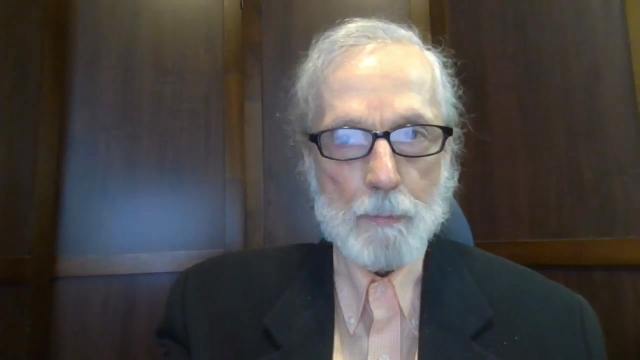 Adaptability is determined by degree and rate of climate change. Climate change is accelerating. the WMO told us, On current policies and trends, we will reach a catastrophic 3.2 c this Century. That's from Working Group 3 and on that scenario, we reach 1.5 c by 2030 and 2.0 c by 2050.. So for all of those that are, 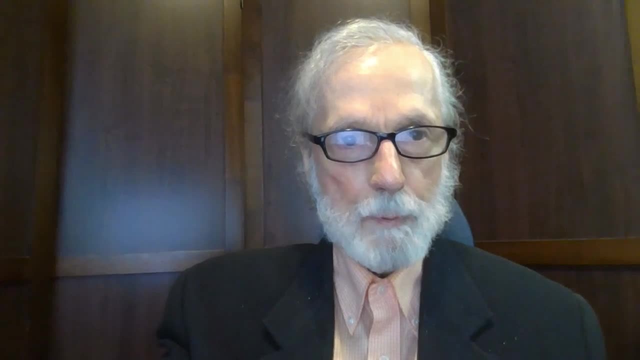 working group 3,. this will be the third or fifth. We have to work our way towards a more planned climate change. The global climate crisis continues to affect each one of us. The global climate crisis is making us more and more vulnerable. We are facing a very serious problem, which is climate change. The two things that we are facing are climate change and climate change alone. 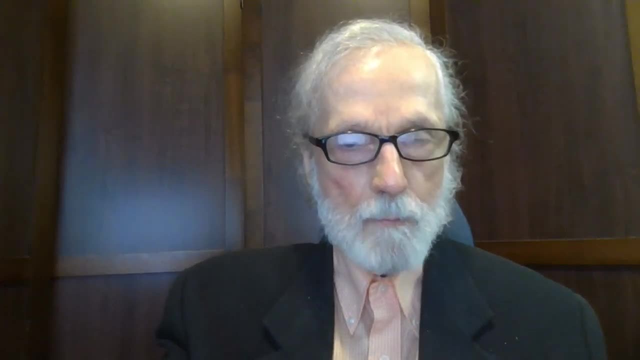 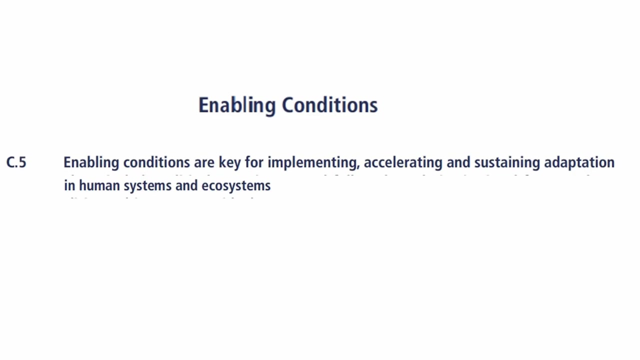 So for adaptation and mitigation for all of us, we must prepare for 1.5 degrees C starting right away, 1.5 C around 2030,. Working Group 2 has enabling adaptation conditions. Extreme world poverty and hunger have to be put right in short order. 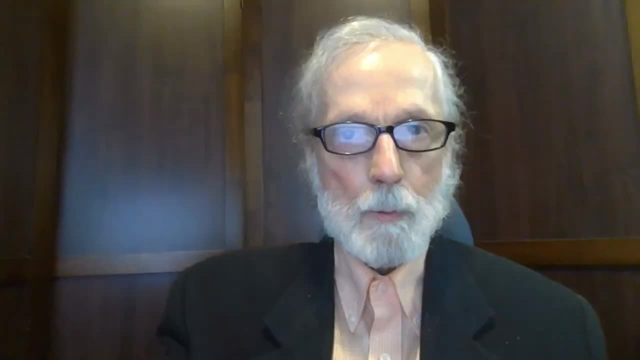 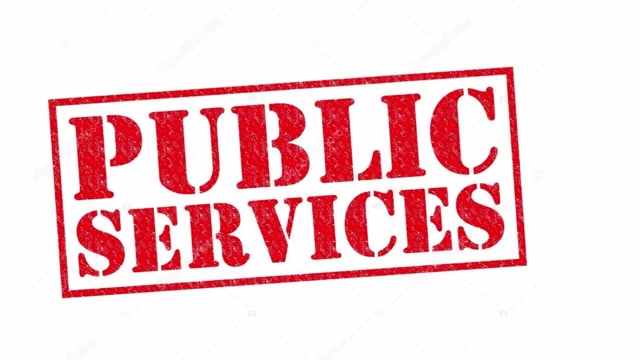 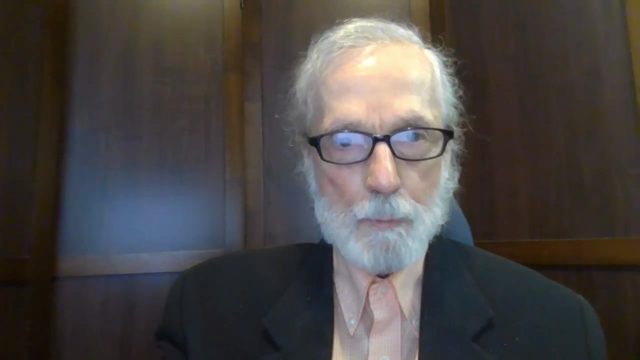 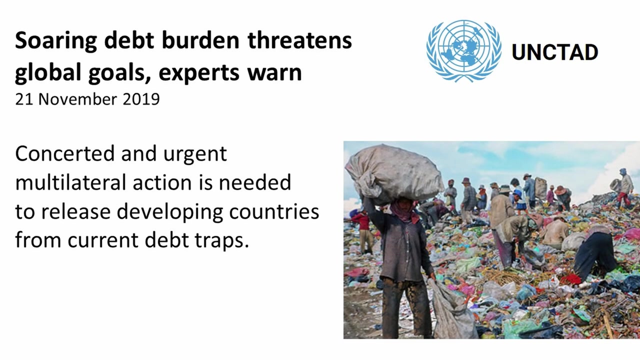 World hunger is increasing again due to climate change and conflict that Working Group 2 say are going together Worldwide development of adequate public services to respond to increasing disasters and diseases has to be started immediately. Debt for already vulnerable poor countries: their debts have to be forgiven unconditionally. 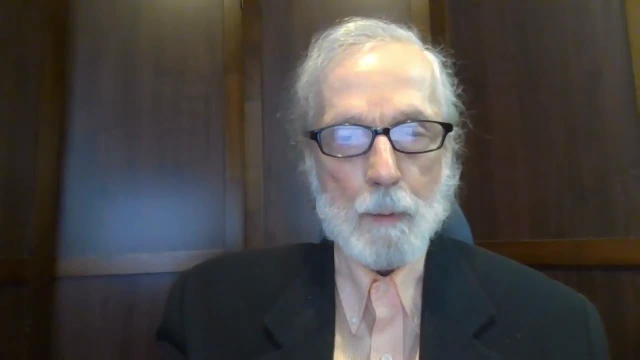 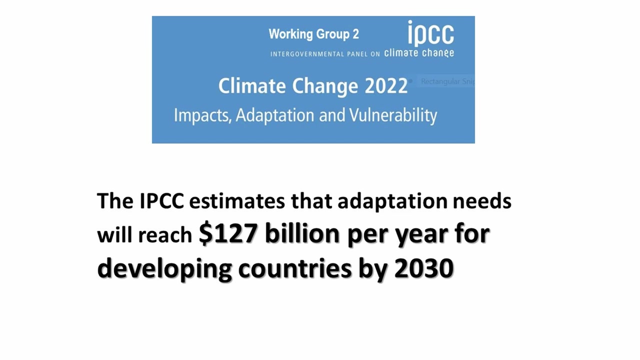 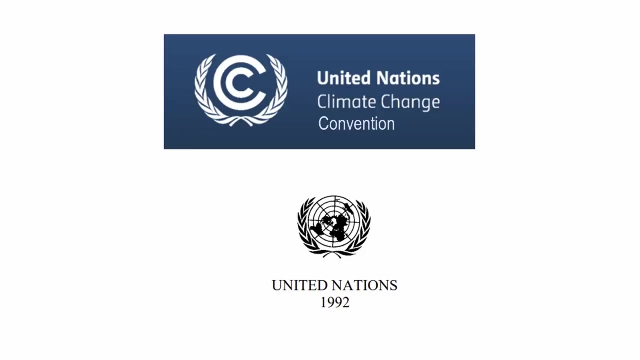 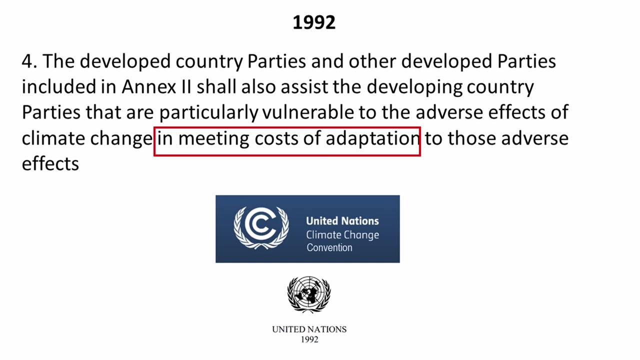 The IPCC estimates for development Developing countries that adaptation alone needs $127 billion a year by 2030.. Of course that's wrong. They need it right away and they should have had it years ago. The 1992 Climate Change Convention said that developed country parties shall assist the developing country parties that are particularly vulnerable to the adverse effects of climate change. 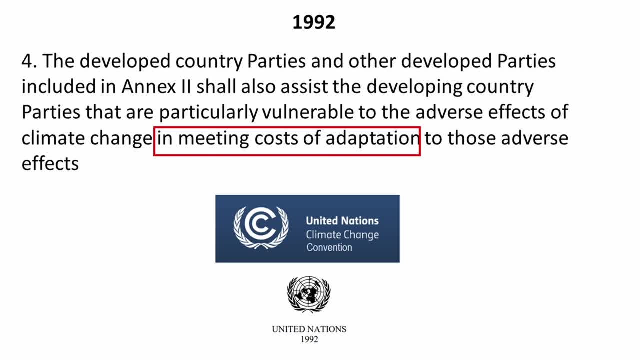 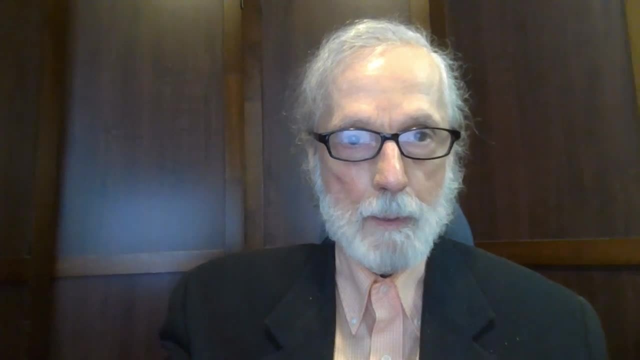 Of course the climate has to be stabilized. That's the top enabler. And for that, immediate global emissions put into decline. For that all fossil fuels have to be phased out, but phased out fast. Fossil fuel subsidies must be terminated immediately, unconditionally. 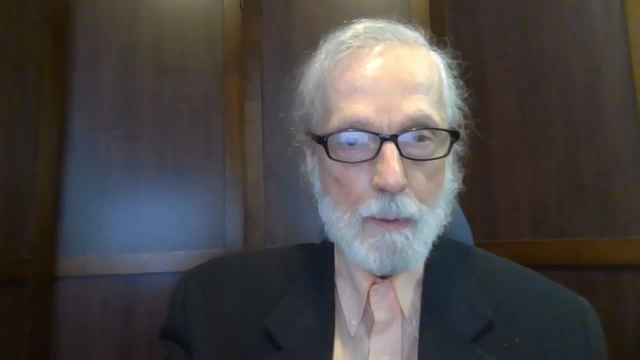 fossil fuels have to be phased out, but phased out fast. Fossil fuel subsidies must be terminated immediately, unconditionally. Working Group 2 says that, to avoid mounting losses, urgent, accelerated action is required to adapt to climate change, while making rapid, deep cuts in greenhouse gas. 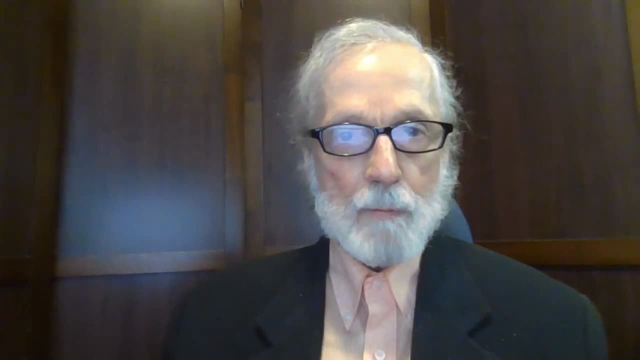 emissions. So I'll close by saying that the survival of many billions of people in the near term depends totally on the immediate decline of emissions globally and then immediate provision, donated, of large amounts of funding for those to develop adaptation. My final word is that that 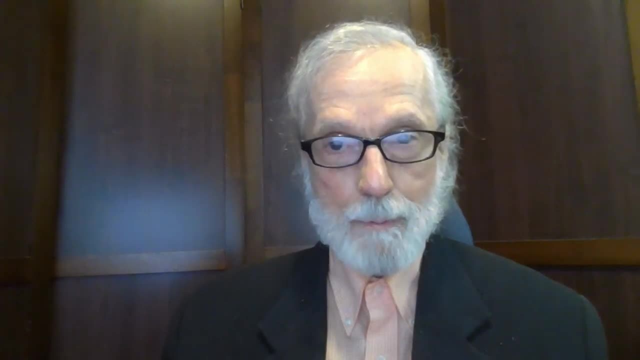 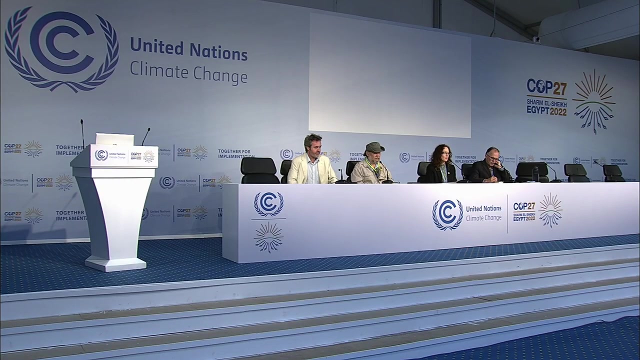 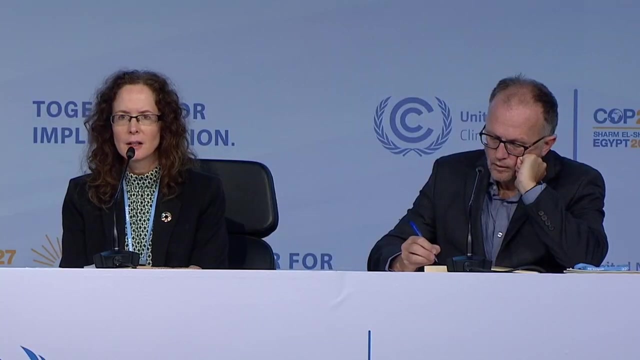 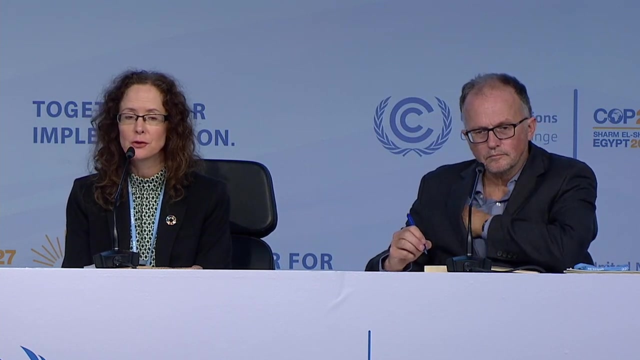 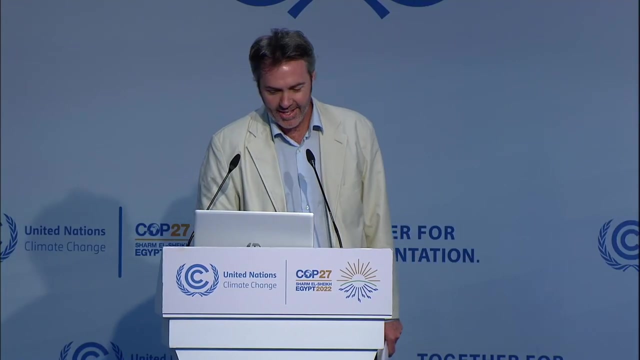 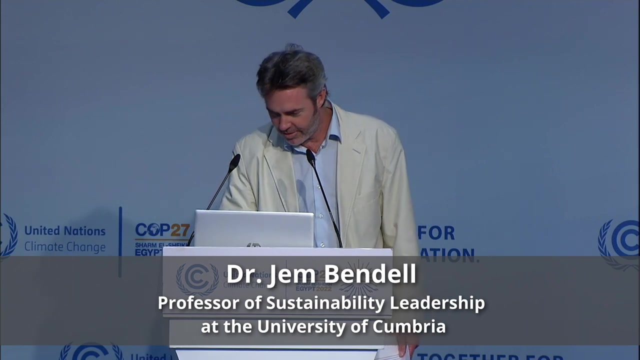 applies to all of us. It applies to everyone in the world. Thank you so much to Dr Peter Carter sending a thank you. Thank you for the invitation. Thank you for coming. We have a communications problem, clearly, because what we've heard is terrifying and yet the world seems to be very good at carrying on as usual. I'm going to speak about that communications problem. 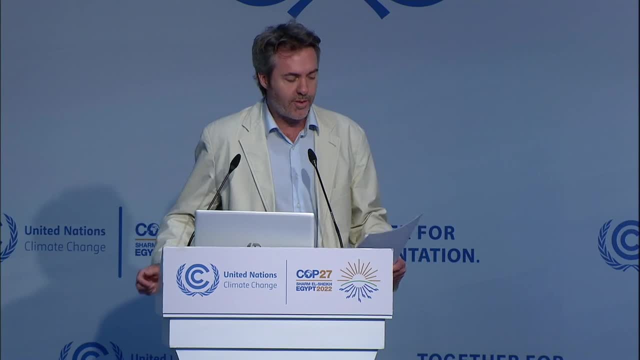 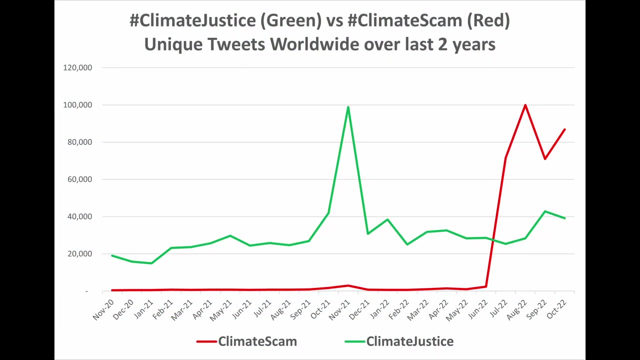 Right now because just as political support for climate action is growing, so political resistance to climate action is also growing. I'm sharing this information for the first time today. The use of the hashtag climate scam has exploded since July of this year, from never exceeding more than 3000 tweets in any month up to June 2022. It's been used 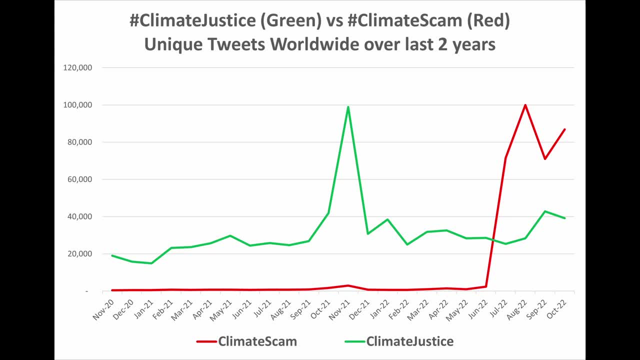 a month in the four months since. Compare that to the hashtag climate justice, which has averaged about 30,000 tweets per month for the last two years and almost it 100,000 unique tweets in the month of COP26 in Glasgow this time last year, what with all the world's. 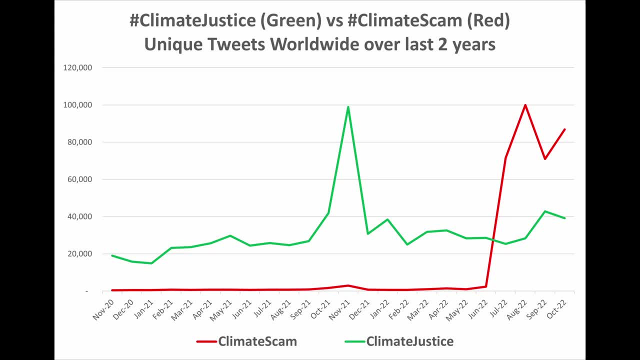 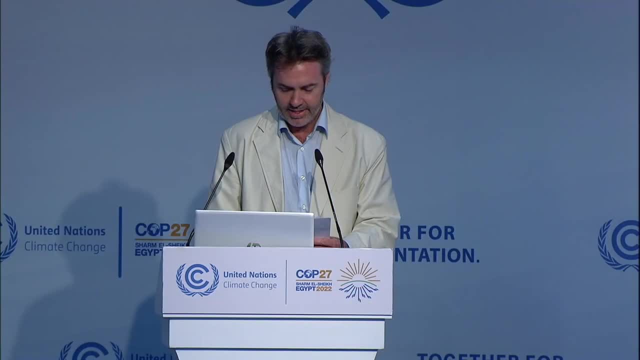 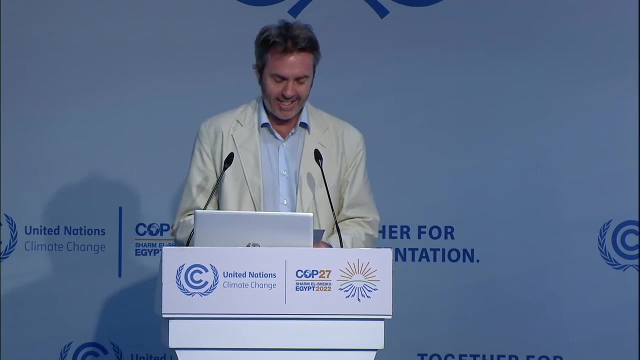 media attention that now climate scam is being used two and a half times for every climate justice tweet throughout the last four months. So these Twitter trends are just one indicator of a growing resistance to climate action. so here at a climate event, we might ask: how can 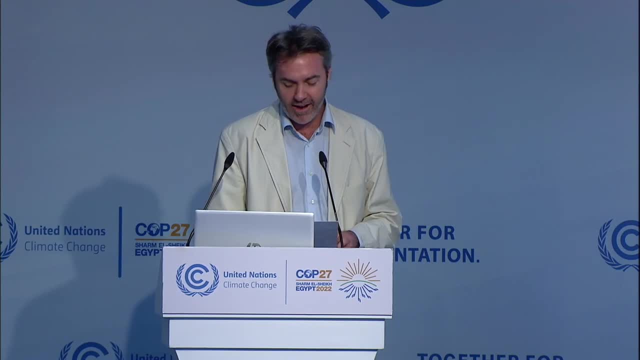 people dismiss something happening before their very eyes. today I'm offering an answer. as a professor and a political adviser who specializes in strategic communications, I assess that resistance to climate action is growing, partly because of the bad way climate issues have been communicated to the public by experts and politicians: badly technical, badly elitist. 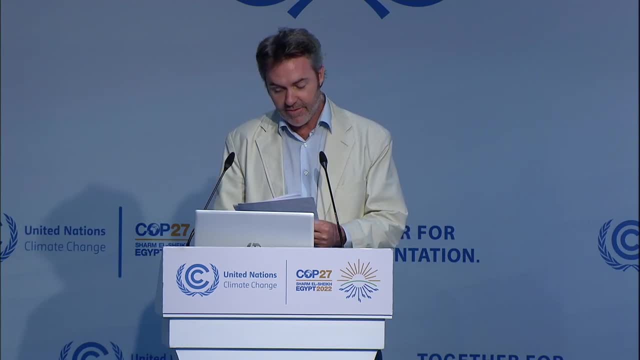 and now badly authoritarian. I believe that reflects a self-serving response from the establishment that's partly to blame for all that current backlash which is represented by this data on social media. so I want to be very clear how I see things. you know, 200 in only 200. 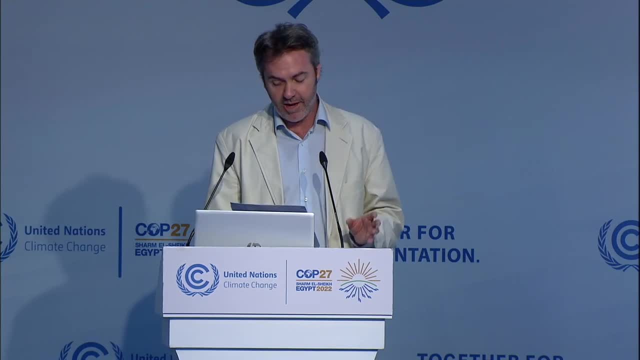 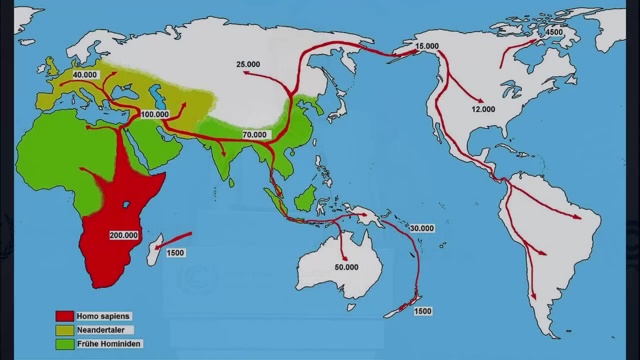 years, industrial activity has increased world temperatures by an amount equivalent to 20% of the total range ever experienced by homo sapiens since we walked on on earth over 200,000 thing, with weather systems already damaging both wilderness and agriculture, let alone settlements and infrastructure. and the speed? that's the crucial thing. the speed is unprecedented. 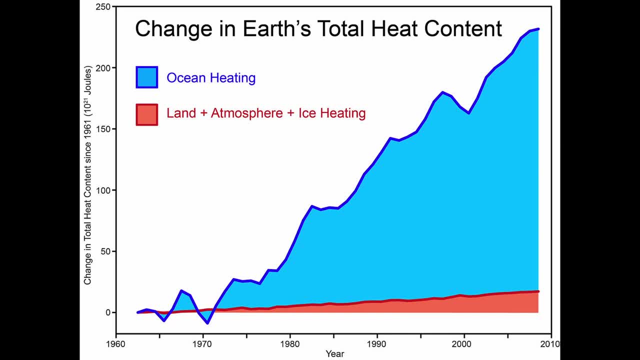 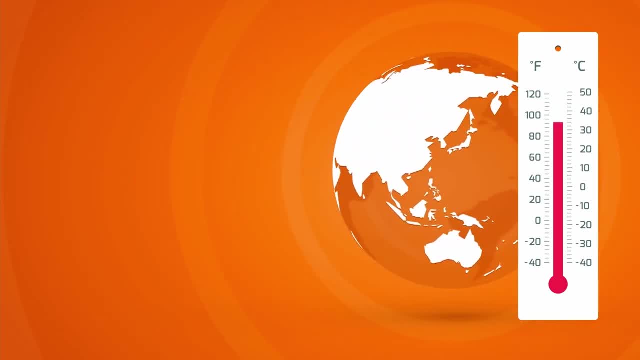 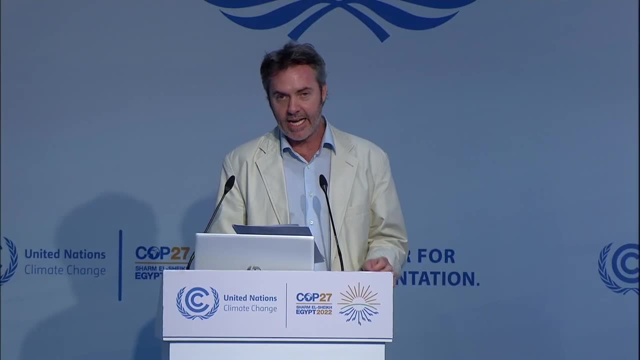 in my 50 years on this earth, our planet's been warming a hundred and seventy times faster than it was cooling for the previous seven thousand years, and that's a speed that ecosystems cannot cope with. Unfortunately, communications about this have been badly technical, using incomparable averages. If the public are told that the world is already, 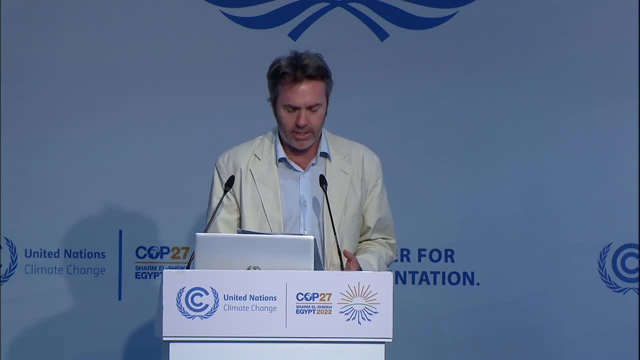 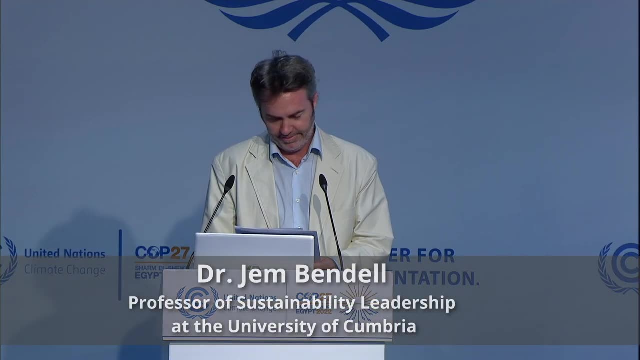 warm by 1.2 degrees. how bad do we expect them to feel? Intuitively, people might think of daily maximum temperatures where an extra 1.2 degrees isn't a big deal. Feelings might shift a bit once realizing that that's an average for night and day, summer, winter. 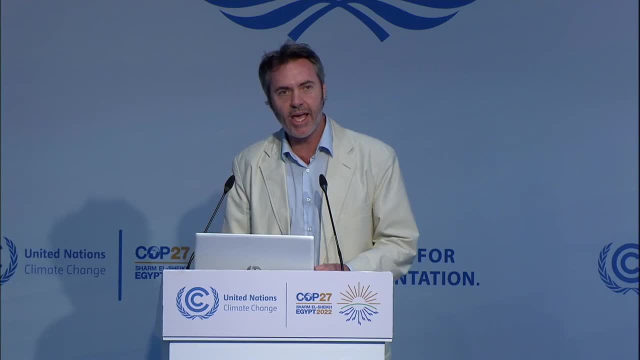 and over land and sea. But still there is nothing to compare that with that small amount, such as by knowing that it was an average of 13.6 degrees back in the year 1850 before rising to our current 15 seas average. So that's a big shift over a tiny period in world. 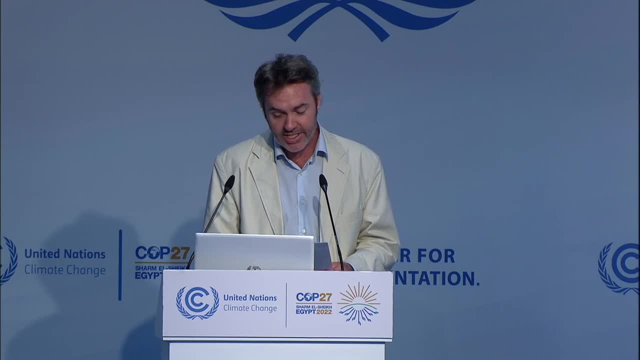 history. But if we're stuck discussing incomparable averages, we will lose to those who dismiss us as wanting to hurt their standard of living for a mere 1.5 degrees, Because in mass communications, once you need to explain, you've already lost. 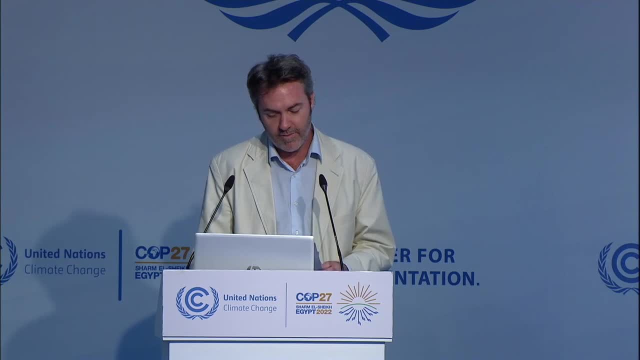 The rush to cash in on the climate crisis that we're now seeing in the halls of this conference is not only generating a backlash, but it's also marginalizing radical critiques. They demand we stay positive, that we will be saved, and saved by technology and saved. 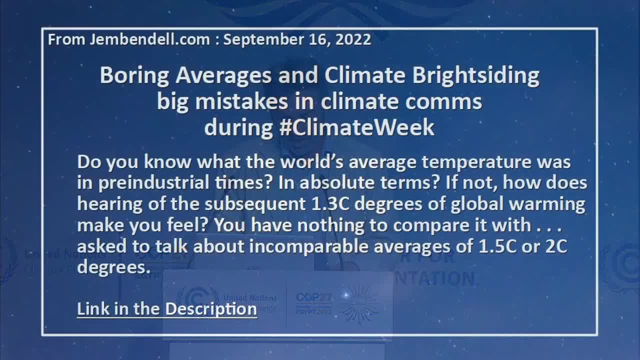 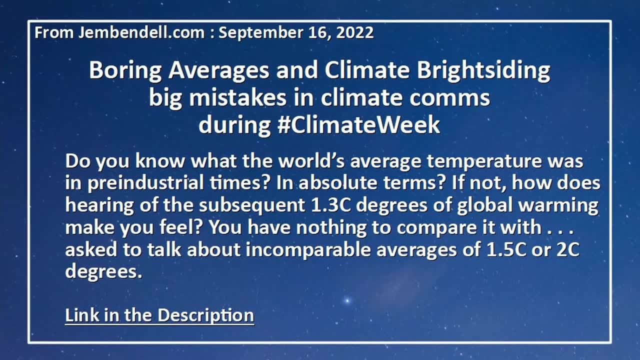 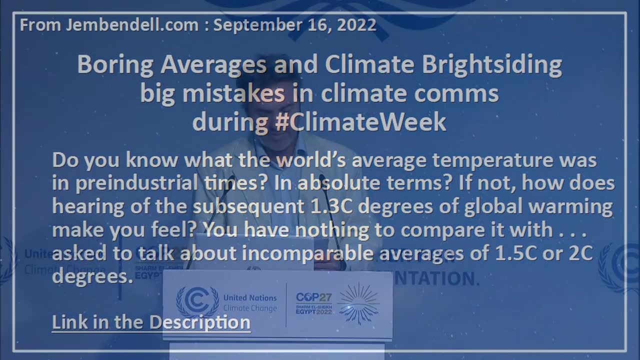 by technology. This is what I call climate bright-siding the public on reality, Because there is some inevitable warming ahead due to how much heat is within the oceans and how much carbon is in the atmosphere. In response, some say that technologies like mechanical direct air capture 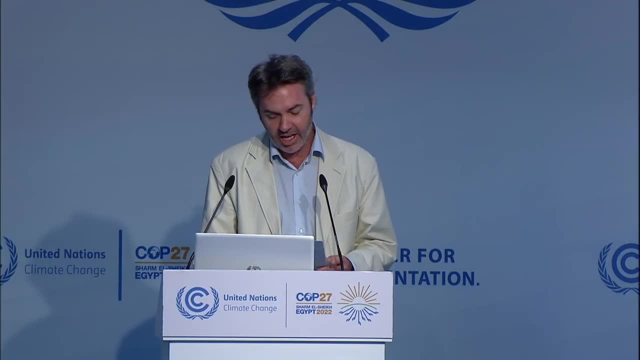 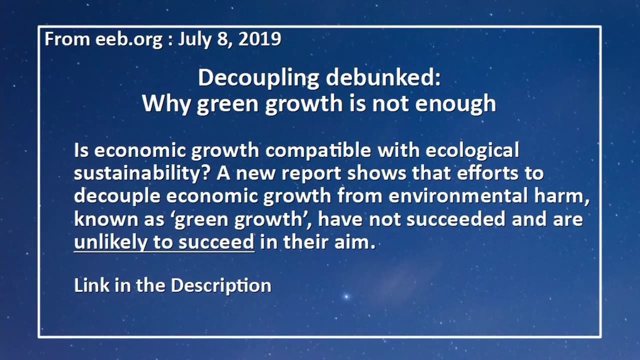 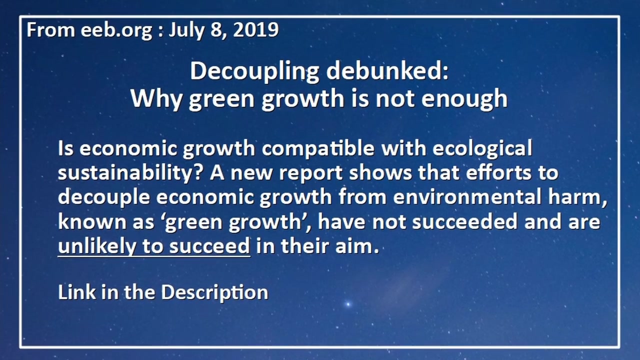 of CO2 can help. However, their low effectiveness and high energy demands should not give us confidence. Meanwhile, research debunks the argument that economic growth can be sufficiently decoupled from resources so that the world economy can keep growing without terrible consequences. 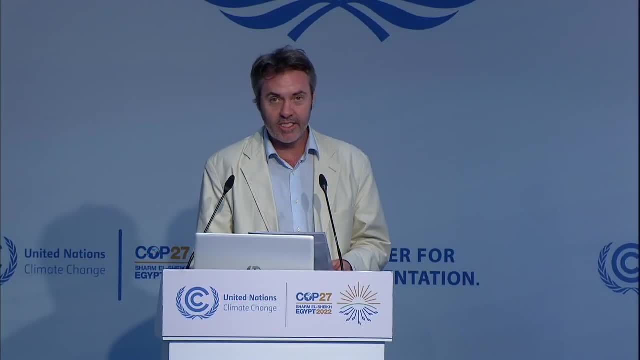 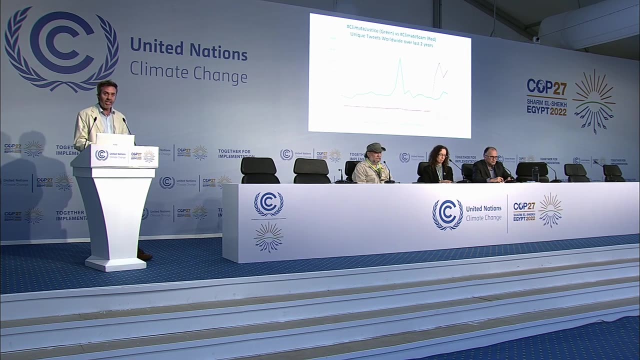 And both psychological research and activist testimony show us that anticipating difficult futures is not demotivating. Instead, believing that technology and big business will sort things out for us is demotivating. But as impacts worsen, atmospheric carbon increases and the science becomes more travel-intensive. 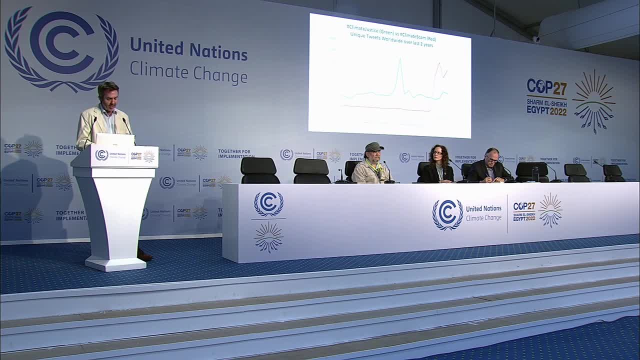 Subtitles by the Amaraorg community: troubling. I think we're seeing a new mistake in how leaders are thinking and talking about climate. Oftentimes, when leaders realize that the systems they administer are threatened, they respond with draconian measures that make matters worse, For instance, brutal approaches. 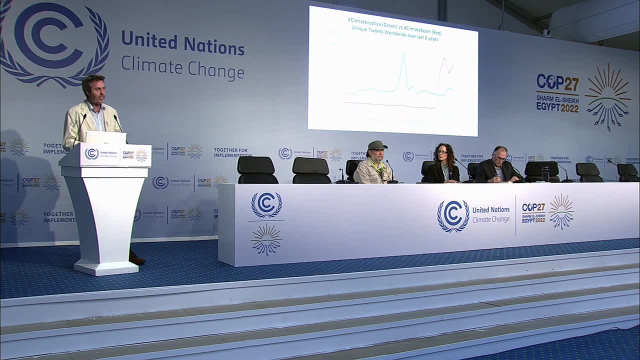 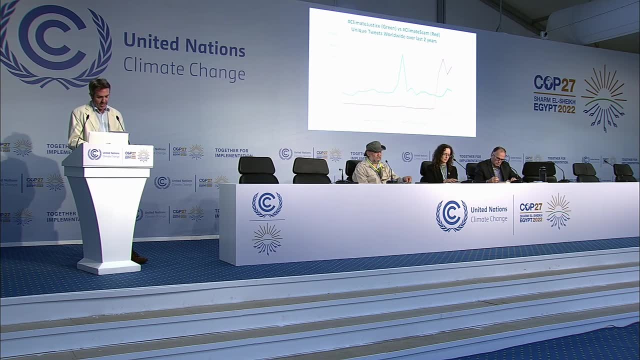 to law and order in the wake of disasters. With climate, such elite panic could inspire leaders to curtail personal freedoms. Resistant populations might then regard action on climate change as synonymous with coercion and coercive power rather than collaboration, And we're already hearing authoritarian statements on climate issues. Instead, the future communications. 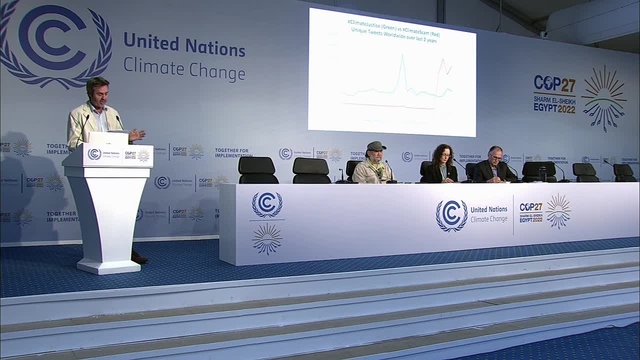 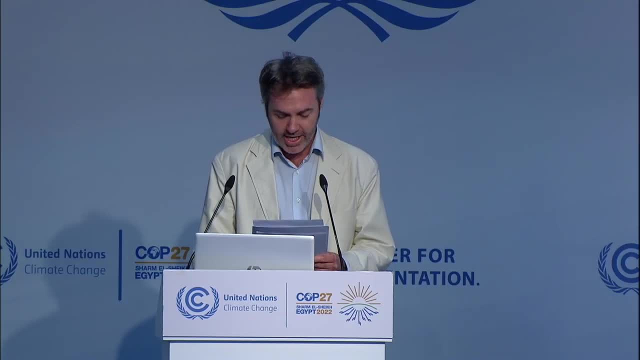 on. this crisis must be focused on freeing us all from the systems that drive us to dump costs onto each other and nature. So let's work with the fact that most people want to do the right thing If they aren't forced by circumstance to do otherwise. So the communications mistakes. 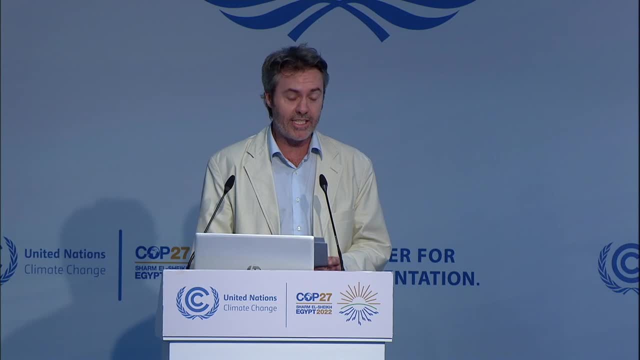 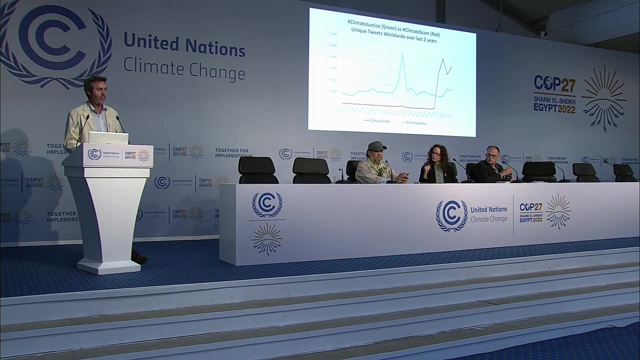 that I've described result from the kinds of people that are currently dominating this agenda, And it's why a bottom up movement on climate justice is going to be central to everything on climate going forward. Thank you, Thank you so much, Jim, And thank you for sharing that startling graphic. It's actually. 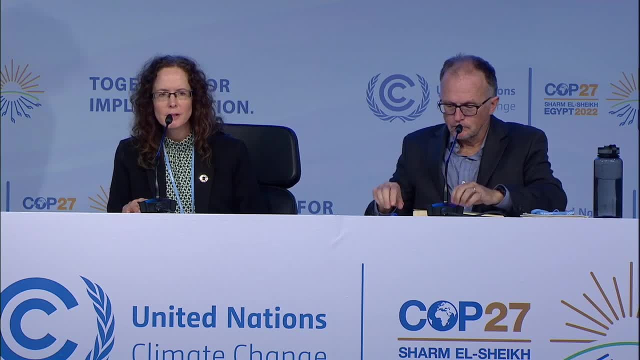 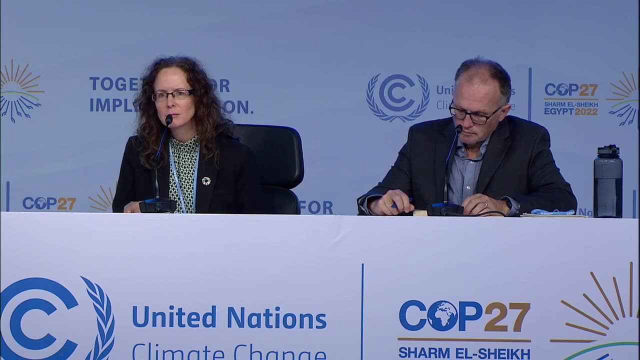 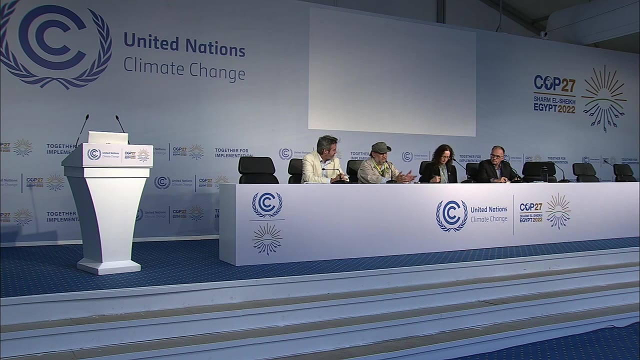 quite frightening. So I'm looking forward to hearing from John Lew some good news. So let's hear what you have to say And I'd like to see- we're going to see- a little video first. Yes, I'd like to thank you all for being here and for inviting me. I'd like to also thank 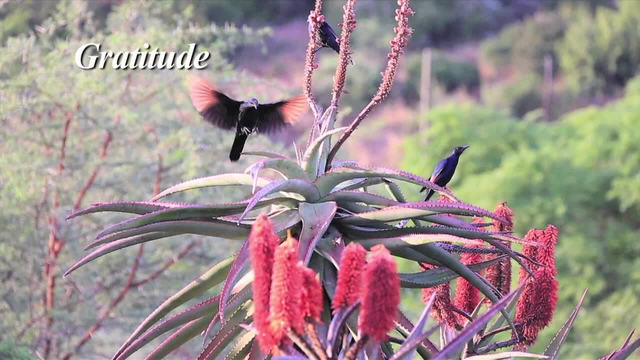 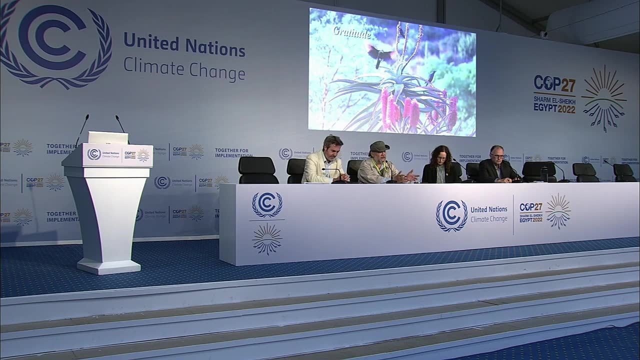 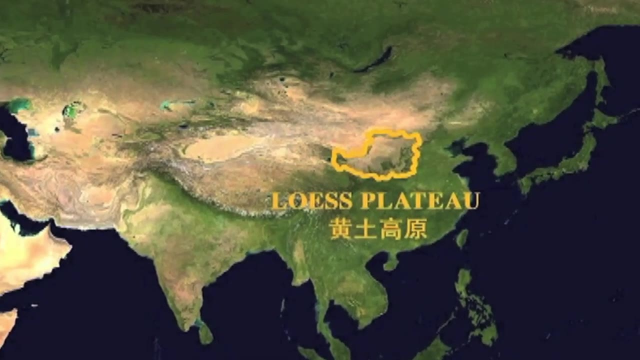 the Common Land Foundation and the Mustard Seed Trust that make it possible for me to do this work. Okay, Okay, Okay, I'm going to go ahead and share that. So in 1979, I went to China to help open the CBS News Bureau, And there I had the opportunity. 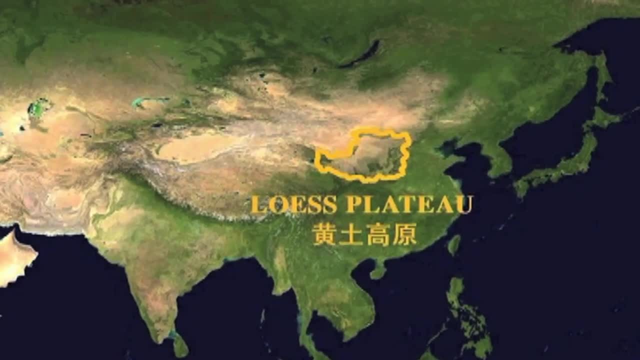 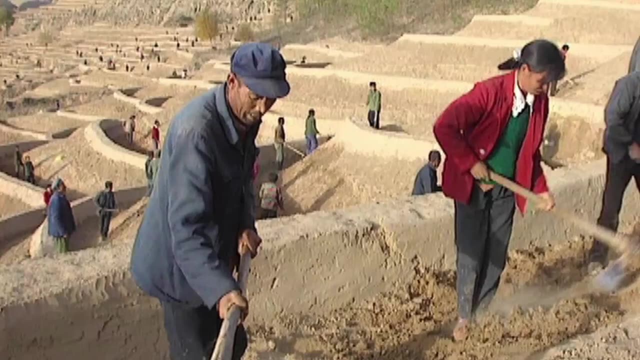 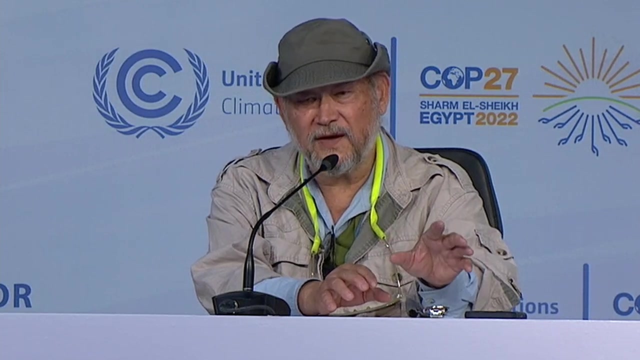 to film the rise of China from poverty and isolation and then the collapse of the Soviet Union. No, just keep going, keep going. You were fine. Yes, This is China's Loess Plateau. In 1994, the World Bank asked me to go there to film. 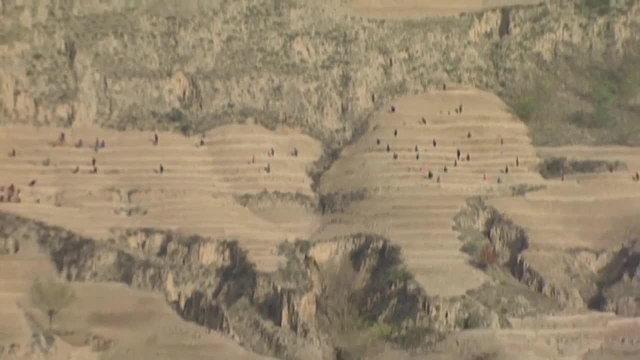 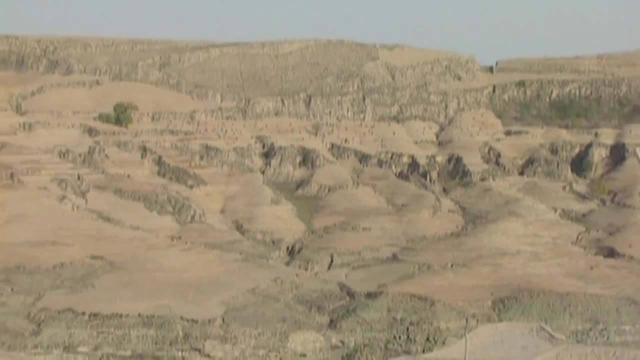 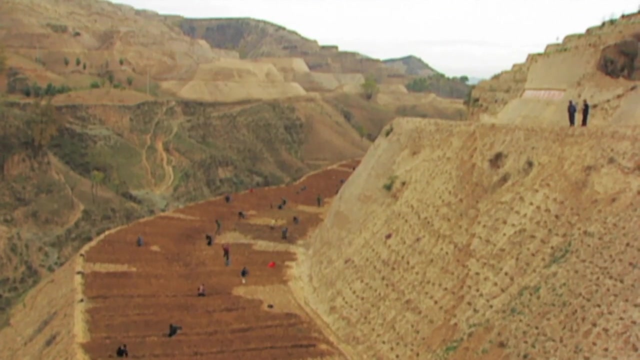 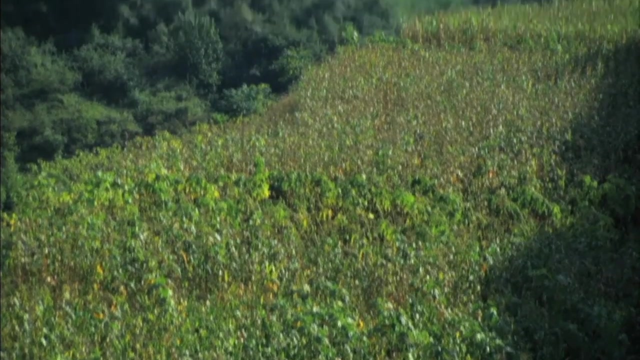 the baseline study, the rehabilitation of this massively degraded landscape. now, basically, they employed the entire population to do restoration, and what's interesting about this it's it was unbelievable to imagine that you could do anything with this kind of a landscape, and they were using their own. 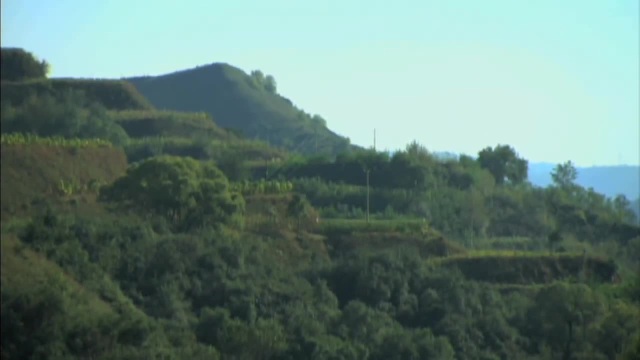 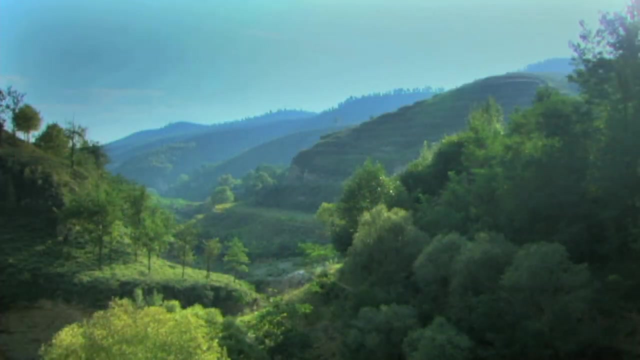 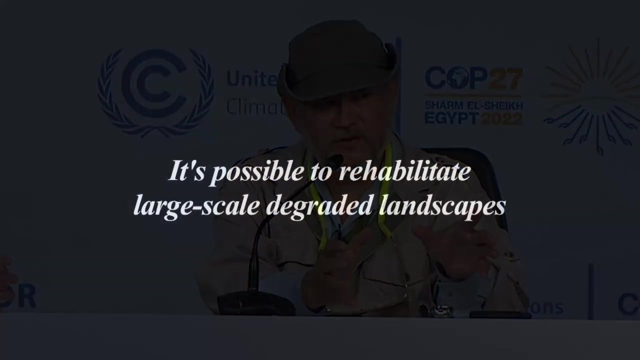 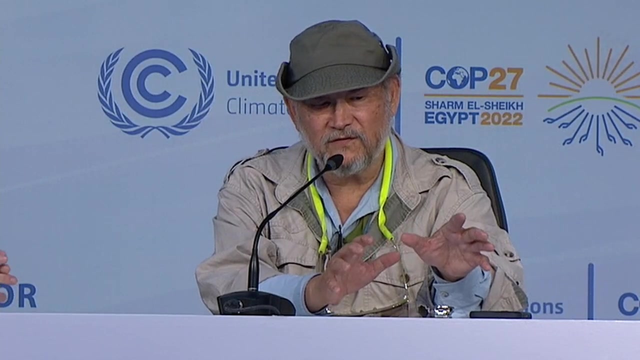 hands and and simple tools. so this is what it looked like when they began and this is what it was able to do in 14 years. so essentially, we learned that it's possible to rehabilitate large-scale damaged ecosystems, including ecosystems that have been damaged over very vast. 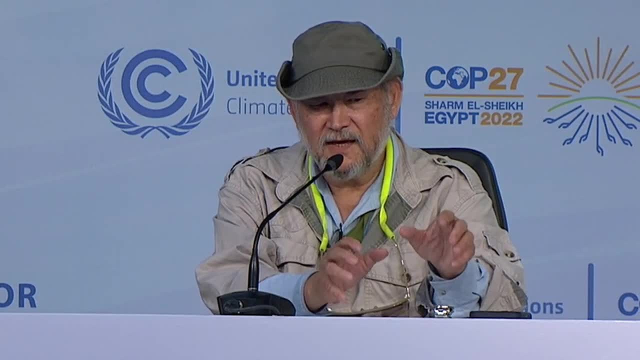 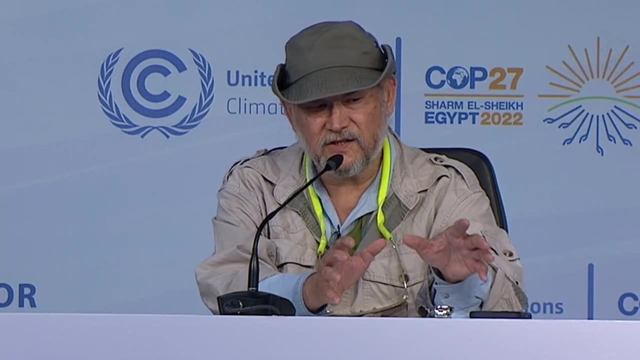 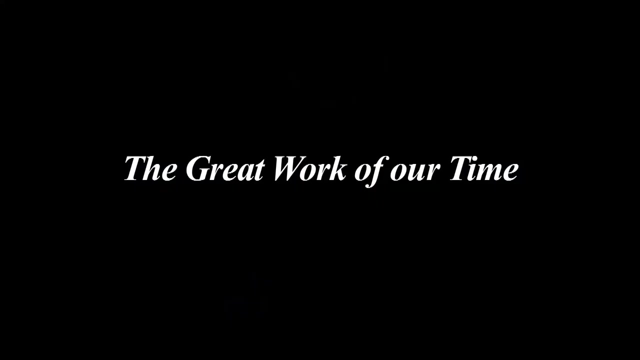 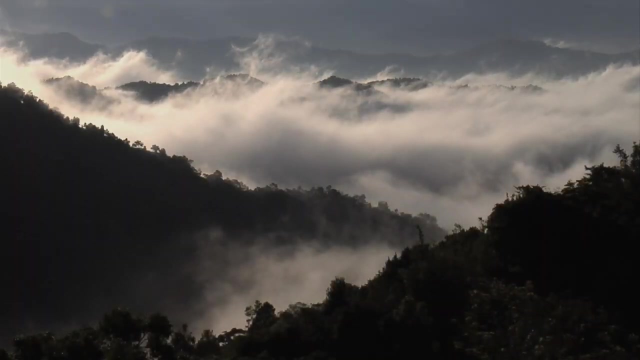 areas and over long historical time. and i began. i stopped doing journalism and i began to study ecology. i've now studied ecology for 30 years in 90 countries around the world. restoration of the earth is the great work of our time. if we choose to do this, we can restore the entire planet. this is the only way that we can actually 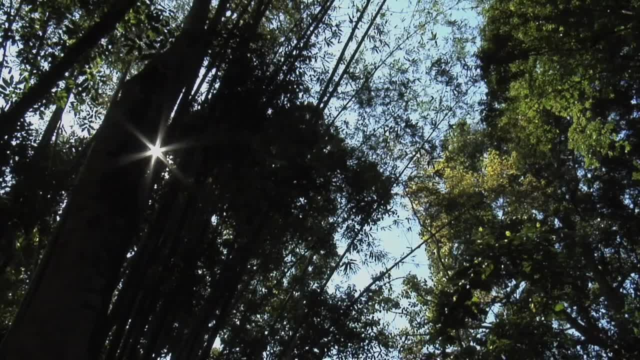 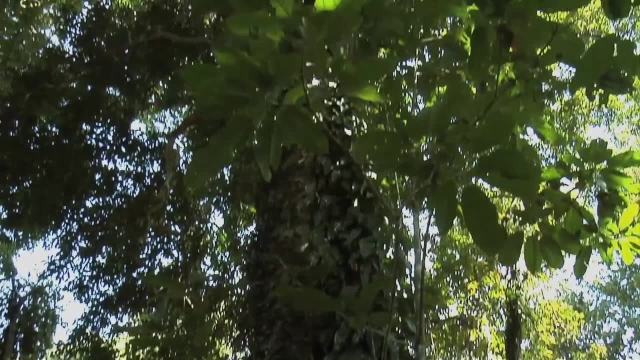 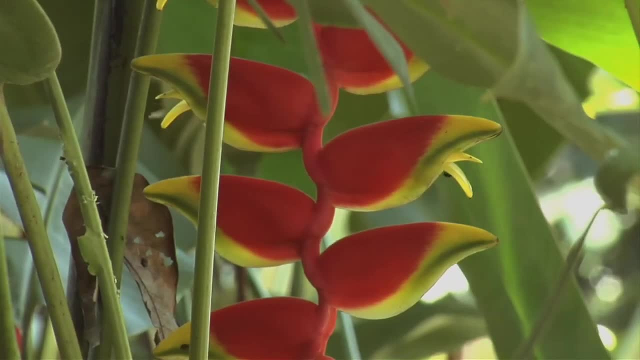 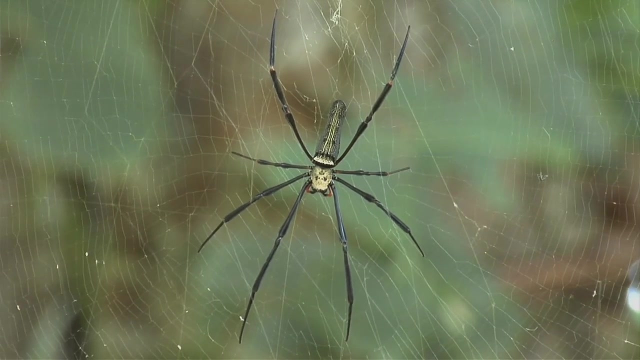 deal with sequestration of carbon, of re-regulation of the hydrological cycle and of controlling extreme and erratic weather events. the principles that i learned in ecology are that there's always more biodiversity, always more biomass and always more accumulated organic matter in natural evolutionary succession. and when we're talking about communications. 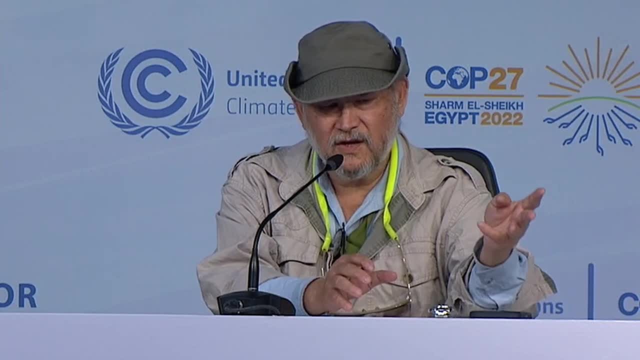 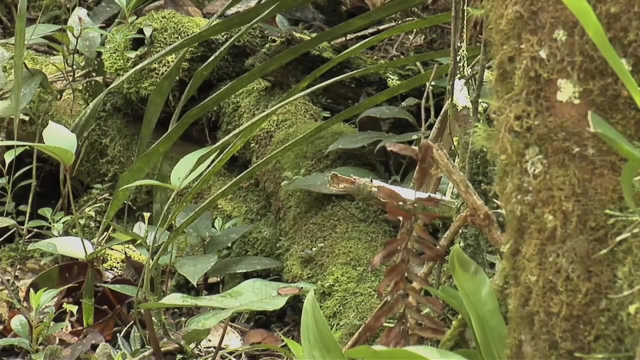 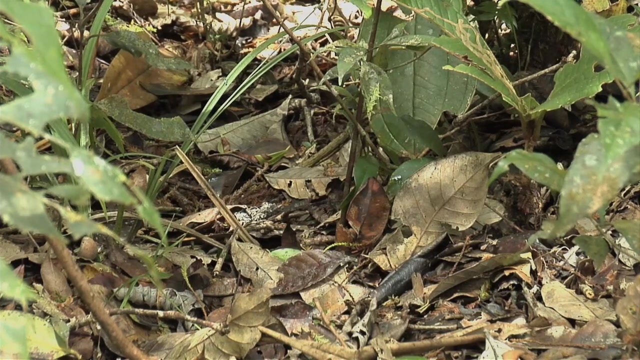 when we're talking about governance, when we're talking about commerce- buying and selling things, we are talking about abiotic systems, materialism. we are a living planet. it's the only planet we know that has an oxygenated atmosphere, a freshwater system, fertile soils and amazing biodiversity. 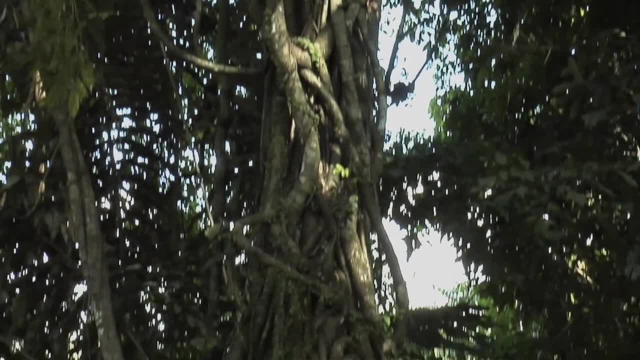 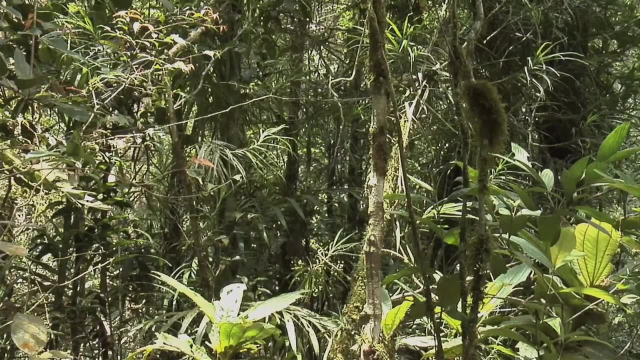 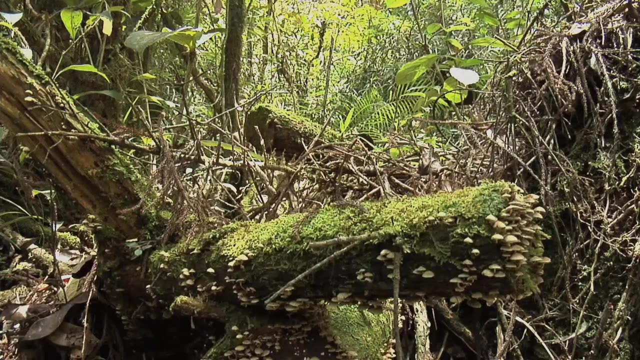 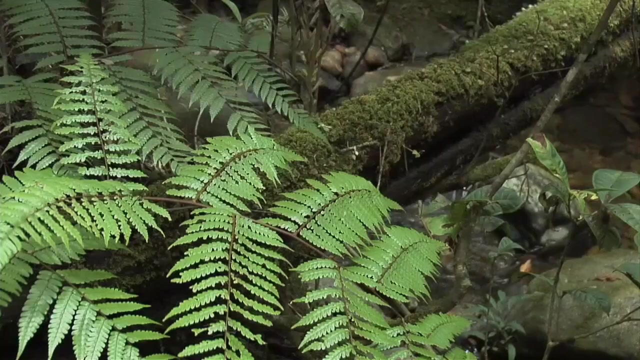 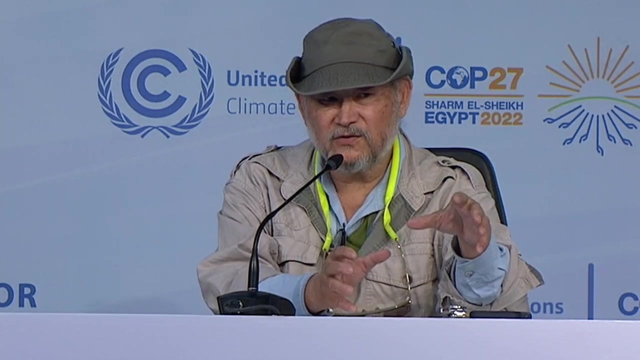 and this is where humans arrived in the garden of eden. and since human civilization began, we have been cutting down the vegetation, we have been destroying the hydrological cycle, destroying the soil fertility, losing the biodiversity, and these are the life support systems on the earth. now this, i want to tell you that we created the ecosystem restoration camps i was having. 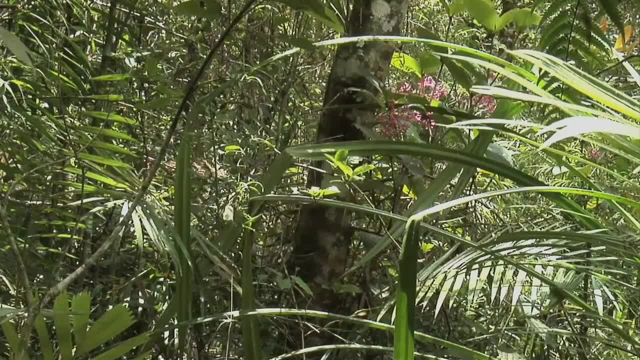 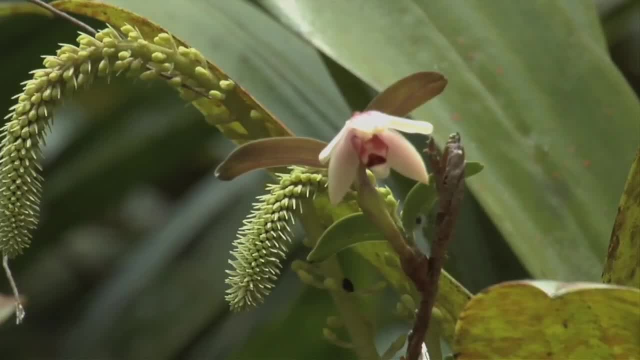 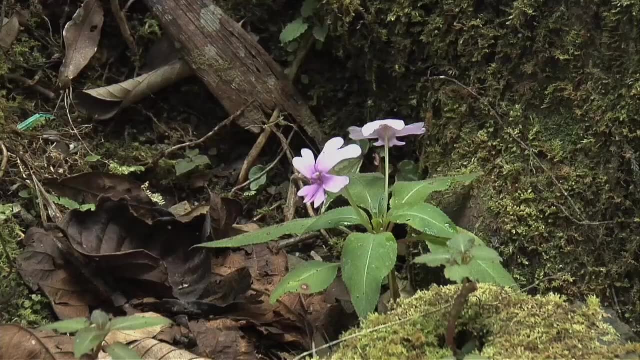 dreams. because i was studying this and i found that i was dreaming about people restoring the earth systems and i had this dream repeatedly and i thought: i'm crazy, nobody's going to do that. i keep making these films and nobody's listening to me. i've been doing this now for 30. 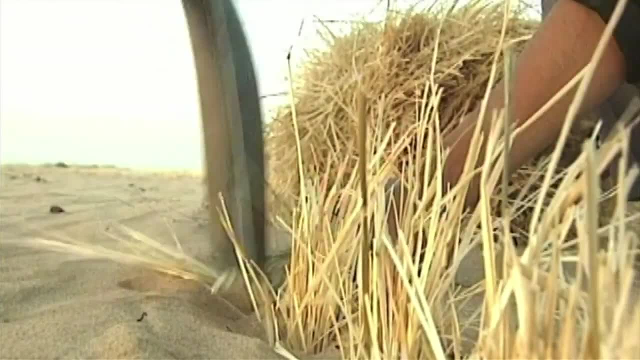 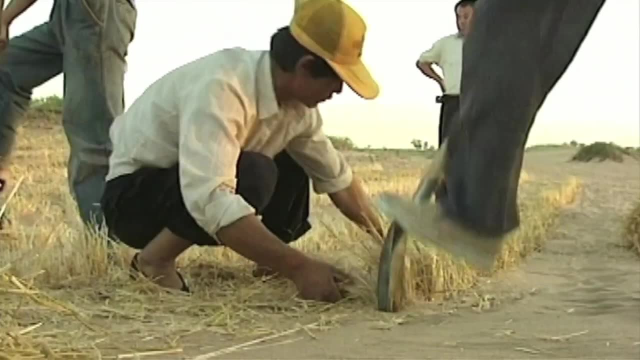 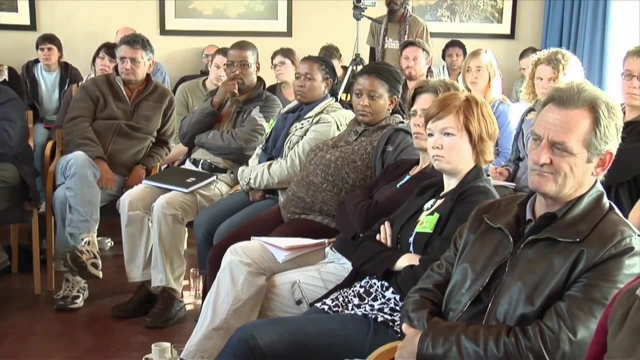 years. so how could this be? but i wrote an essay called earth restoration, peace camps, and people began to show up. tens of thousands of people said: that's what we need and that's what we want. this is a bottom-up movement. that's what we need and that's what we want. this is a bottom-up movement. 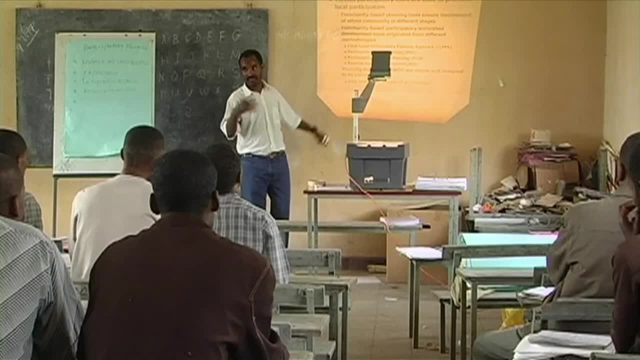 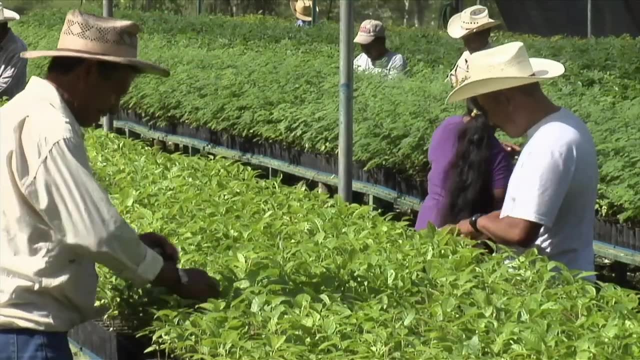 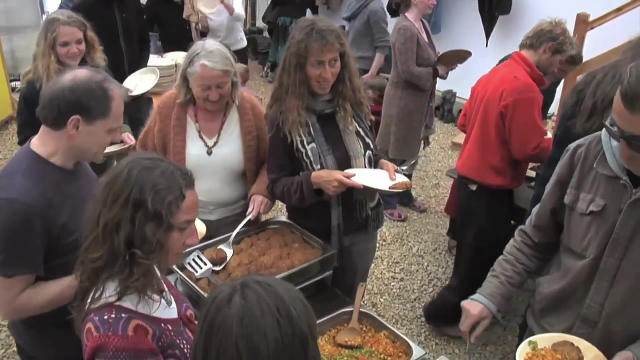 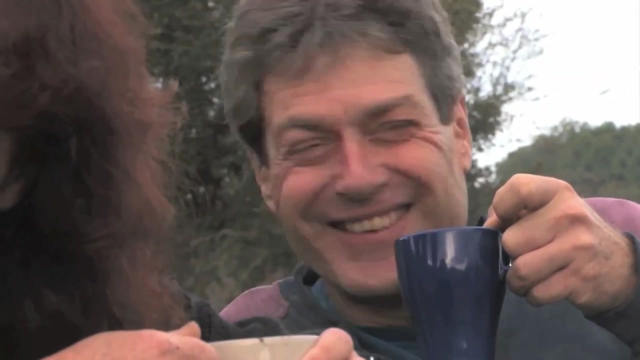 that is working all over the world in six years. there are 55 camps in six continents. so in these camps it's possible to restore the hydrology, restore the soils, restore the vegetation, and not only that, but it ensures food security. we're recommending all of these places have central kitchens, creator spaces and cultural stages so that, as 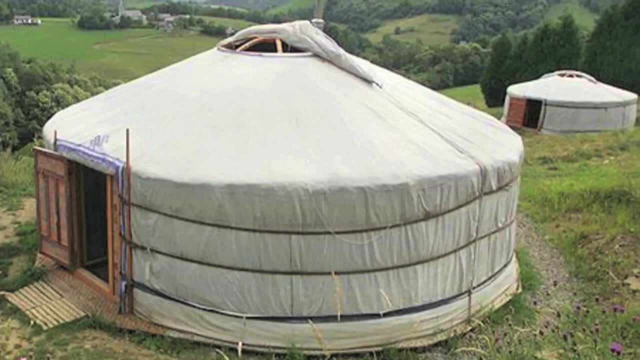 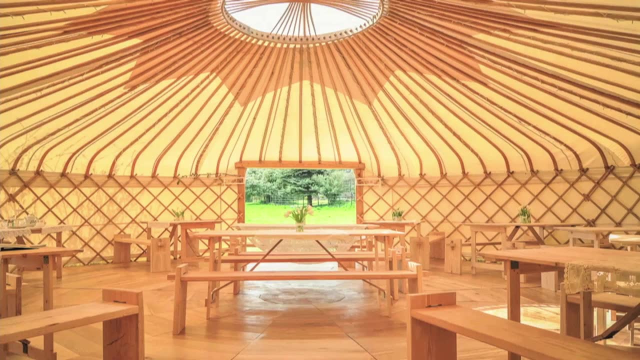 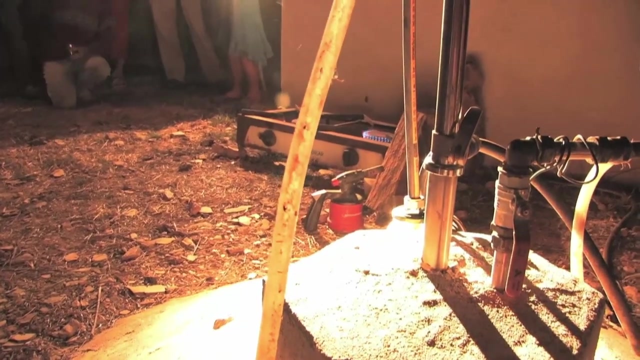 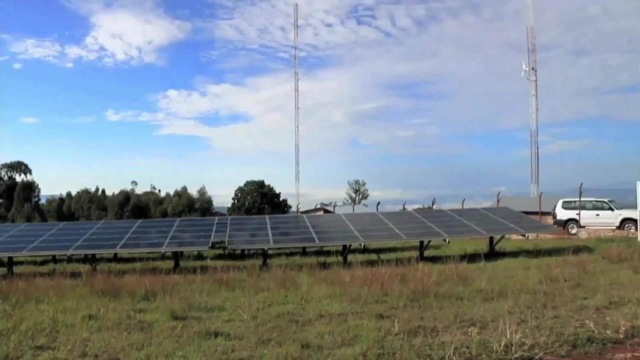 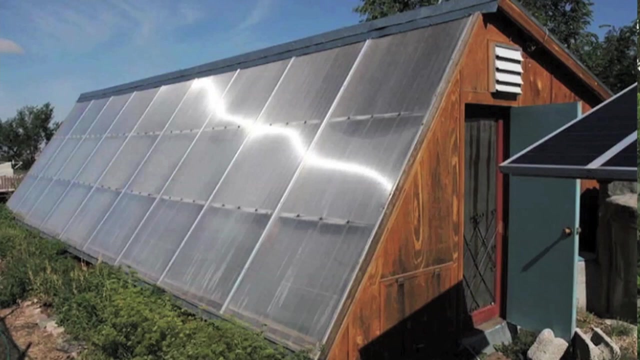 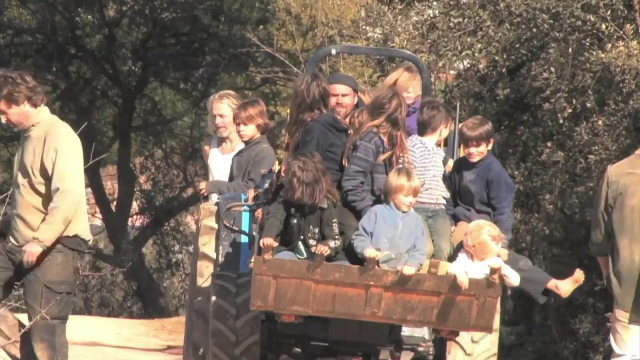 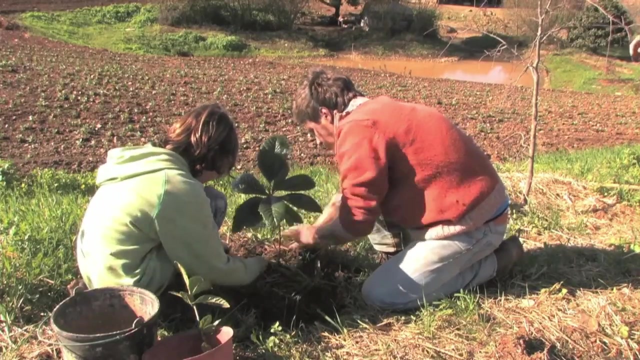 well as the take care of everyone, so that really no one is left behind. and if we get this right, we apply it to the refugee situation, to the homeless, to the hungry, because they have the same rights and the same energy that if we use it and they participate, we all participate, we will live. 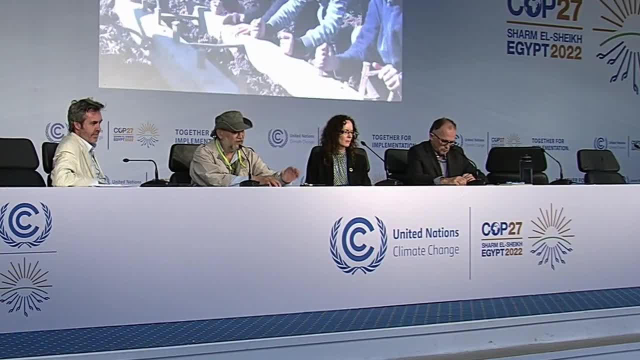 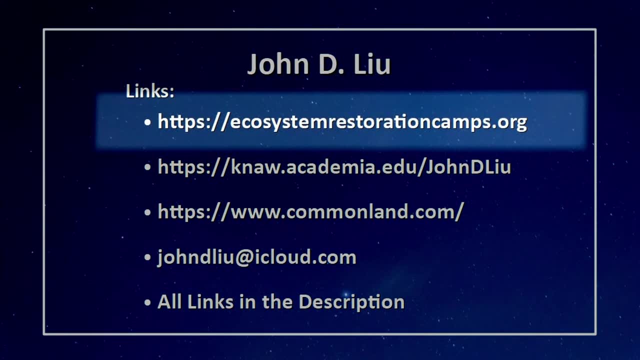 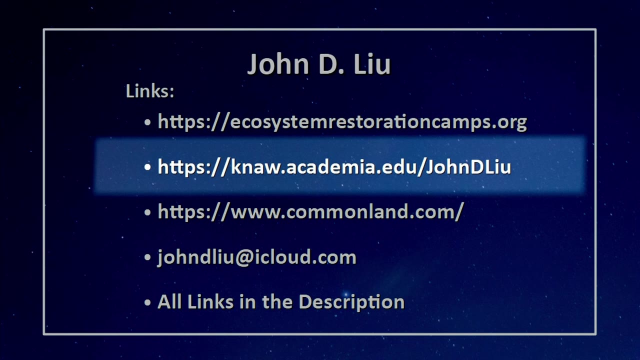 and take care of one another, we'll be safe, we'll be fine. so I highly recommend that you look at ecosystem restoration campsorg if you're interested. I have dozens of films I've published on the BBC and on National Geographic and and all over the television stations. my writings in 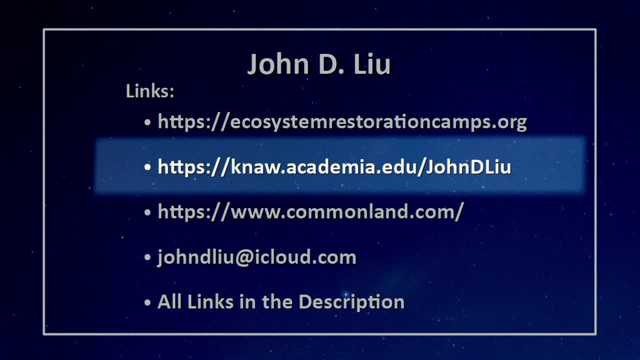 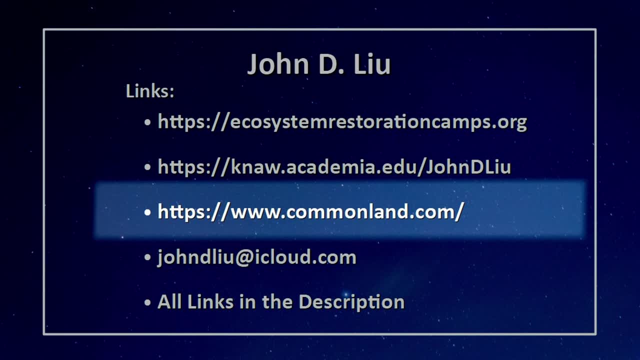 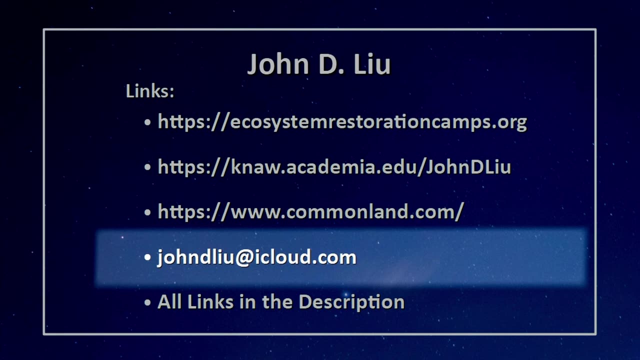 journals are also in there on this, this thing. Common Land Foundation has two million hectares in restoration as well- ecosystem restoration, campsorg- and that's my email. I'd love to talk to anybody who's interested. thank you very much. thank you, John. I have to say that was quite inspiring. that's one of the 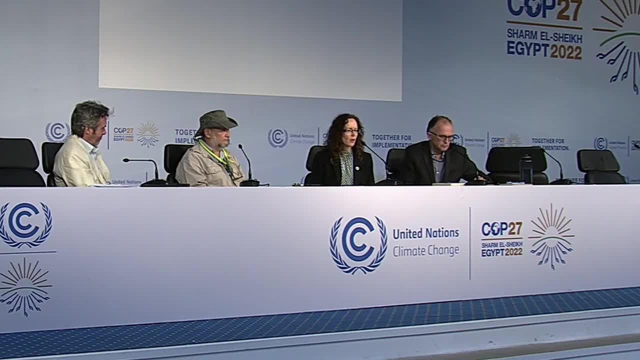 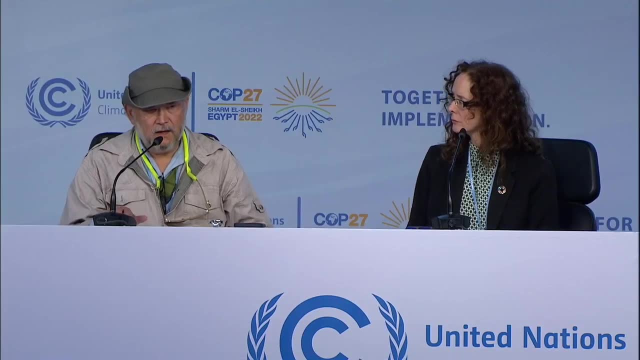 more inspiring um talks that I've heard so far in the cop. and just a quick question: is this a type of camp or people could go for a few weeks, or how does that work? each camp is autonomous, self-organizing and self-governing. they're based on what the community needs and 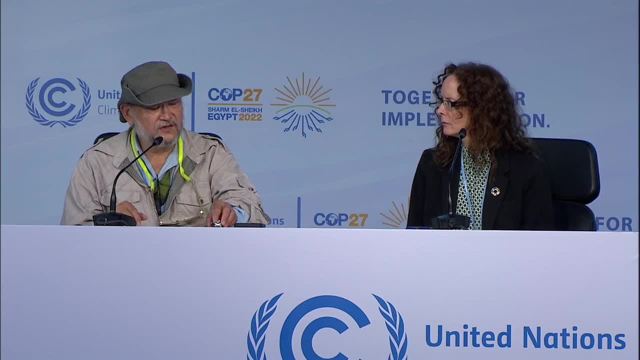 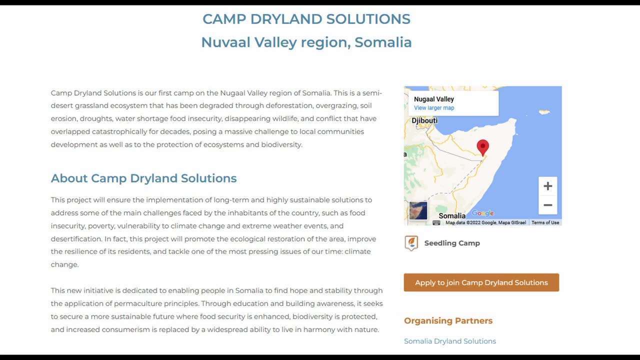 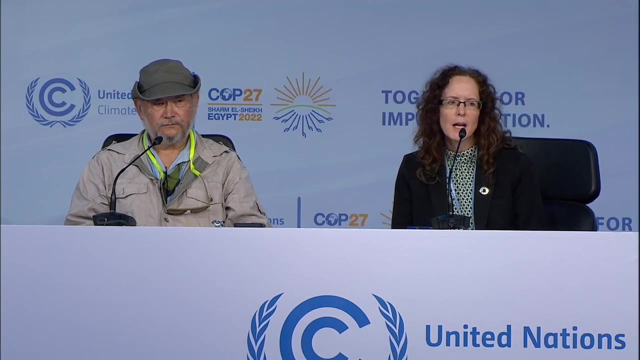 wants I. I'm working on one, especially in Somalia, that we think is going to become- uh, it's called dryland Solutions, and I think it's going to be a model for places all around the world. well, thank you so much, so, very, very inspiring, wonderful work, and now I'm going to pass it over. 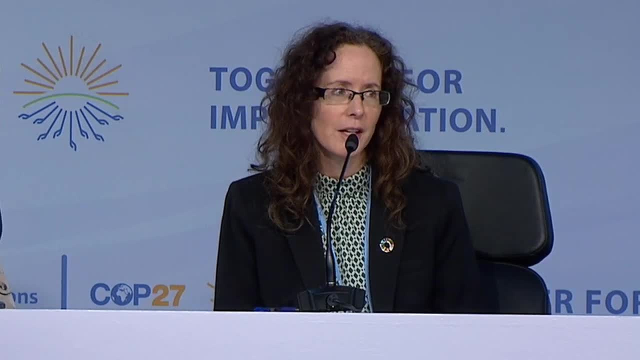 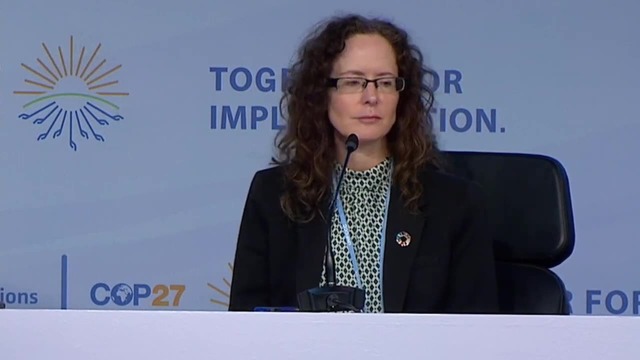 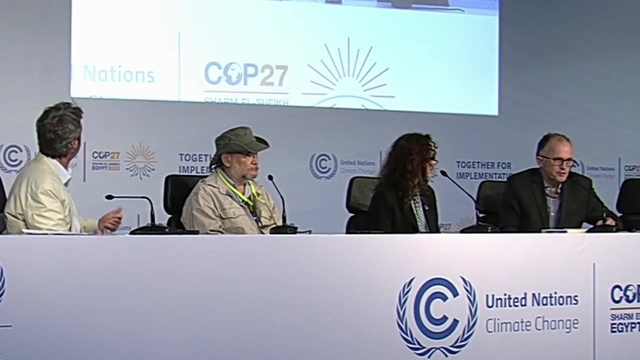 to Paul Beckwith. as mentioned, Paul Beckwith is a climate science educator, so I'm ready to be educated. thank you, and uh, I'm sure many of you have seen uh the before and after images of uh glaciers, for example, a picture of a glacier from a hundred years ago and a picture of that region now, um, which is basically. 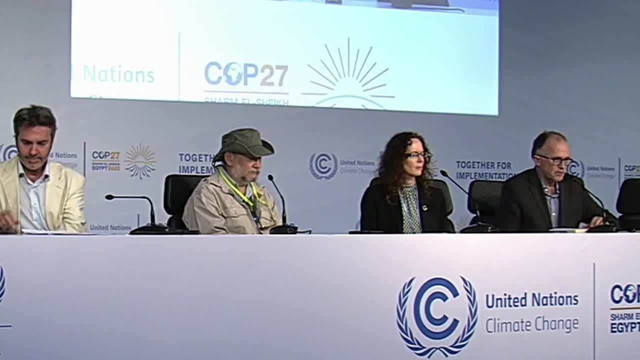 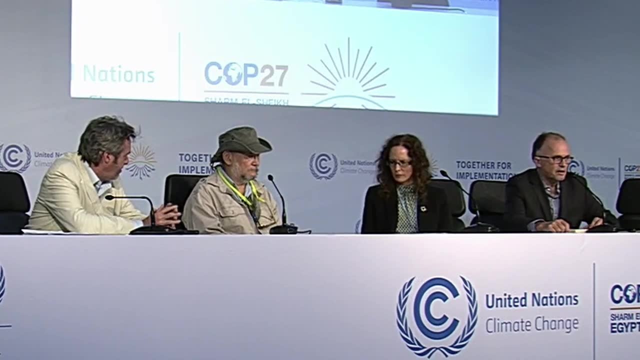 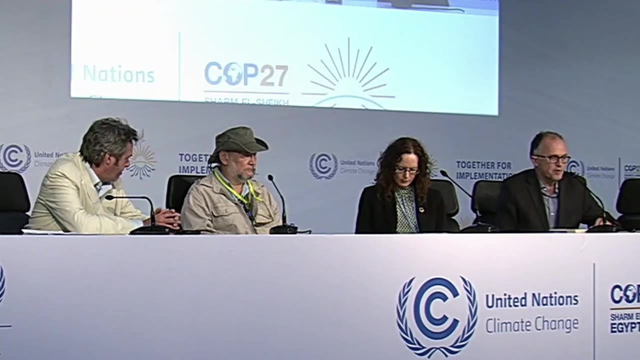 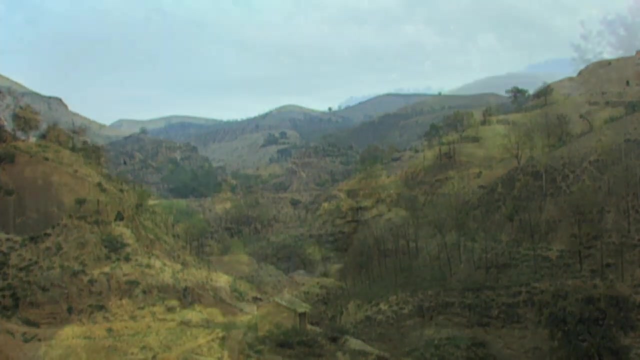 bare rock. well, the uh image that uh John just showed of the, um, you know, completely barren landscape and, uh, you know how, over time, without any human intervention, it would eventually maybe restore itself. maybe not, but with human intervention, smart human intervention, um, clearly, uh, you know it greet, the whole area was greened. it's just, it's just a striking before and after photo. 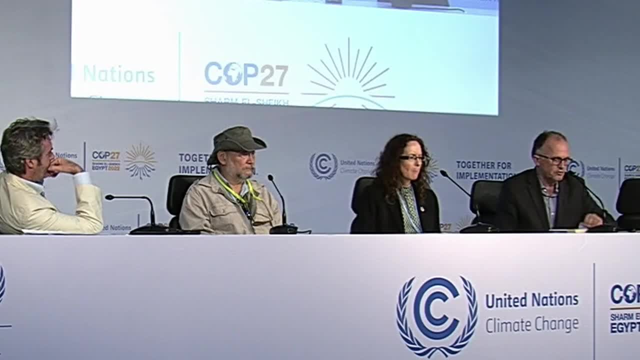 um, but of the good kind, not not of a glacier disappearing. so that was that was incredible and uh, you know Jem was showing that image, the uh plot showing um that we we have a problem with uh social media still and communication. there's far too many climate deniers who are um impeding process at all levels and it. 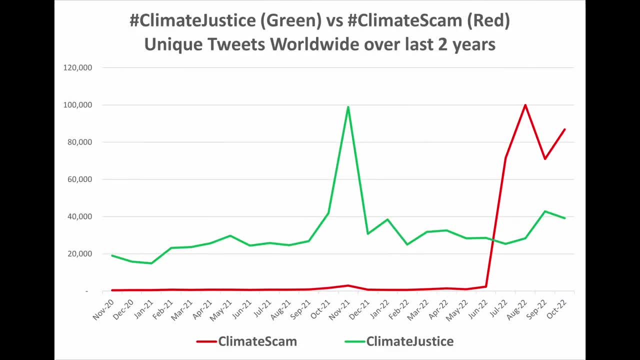 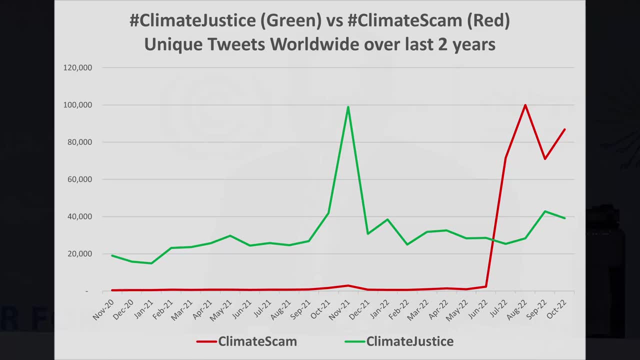 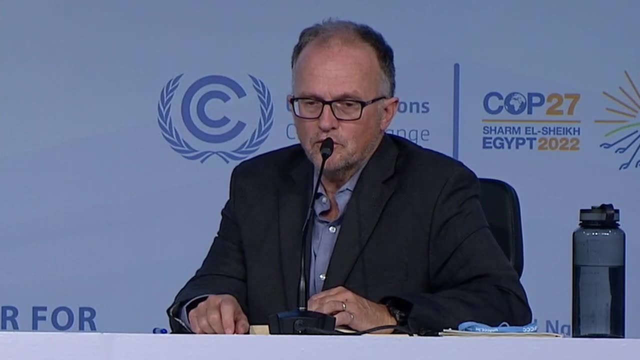 seems to be getting worse, as he showed in the last few months. uh, you know, with the climate scam hashtags and uh, we see a lot of things going the wrong direction. we should be making progress on um restoring the earth, um reducing CO2, things like that, but we're still not anywhere close to doing. 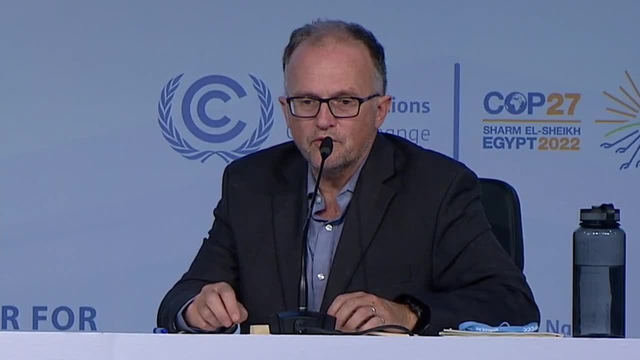 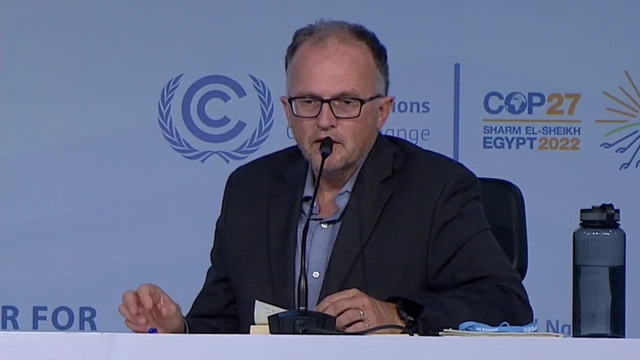 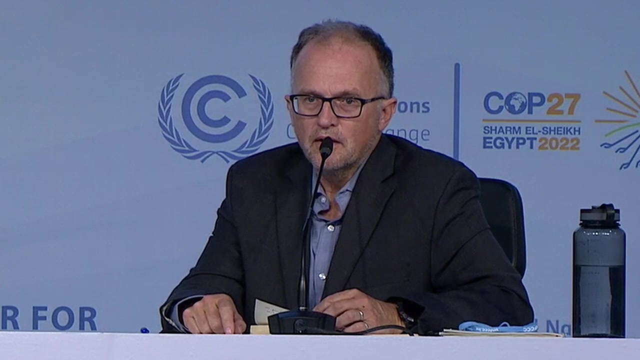 that these conferences, these COP conferences, and you know, are we really making any progress? it's questionable. so you know the number I look at as from a science point of view is the greenhouse gas concentrations. so once again, we're setting new records in greenhouse gas levels, of both of co2 in the atmosphere. 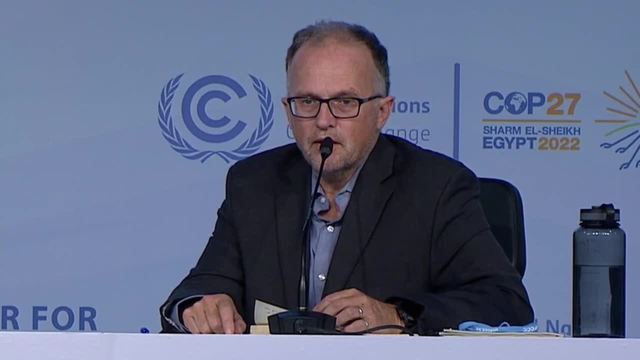 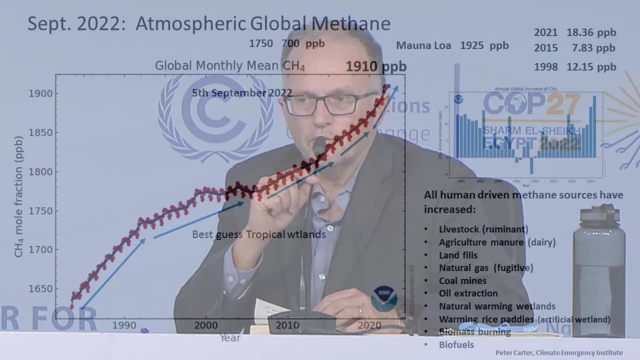 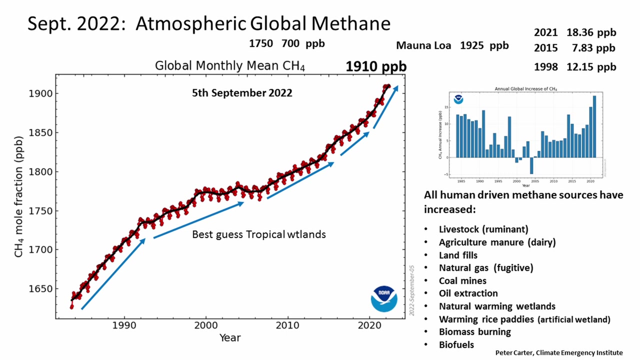 of methane, of nitrous oxide and you know, lately scientists have been making a lot more noise about the methane levels. because methane levels are just shooting up, they're accelerating and perhaps a hydroxyl sink which removes methane from the atmosphere is maybe weakening. we're not sure, but there's a frightening rise. 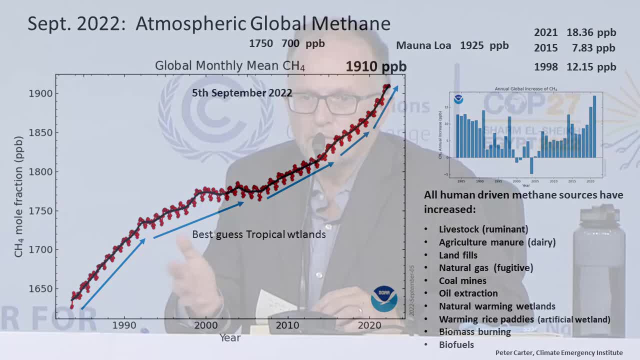 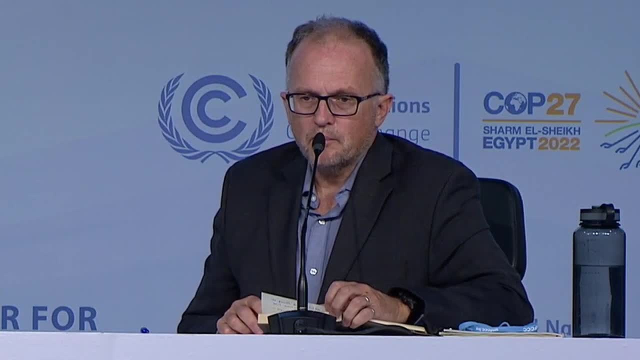 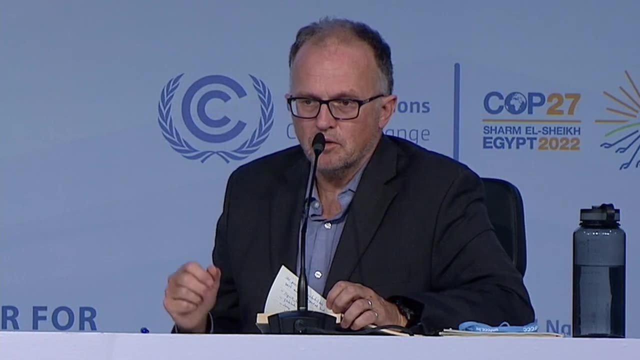 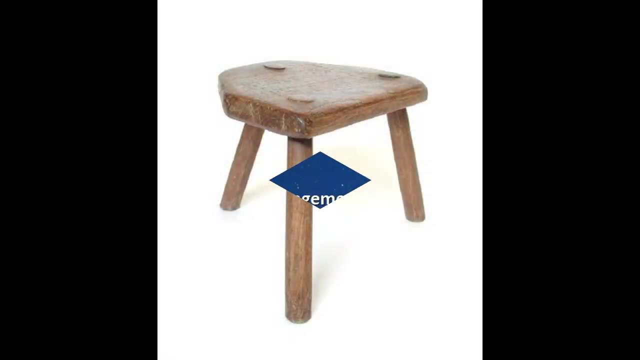 of methane concentrations in the atmosphere, so all of these powerful greenhouse gases are trapping tremendous amounts of heat. you so, when people talk about solutions, of course the nature-based, natural methods are just brilliant, like the work that that John is doing. I've always talked about sort of a three-legged approach or three-legged bar stool where we need to. 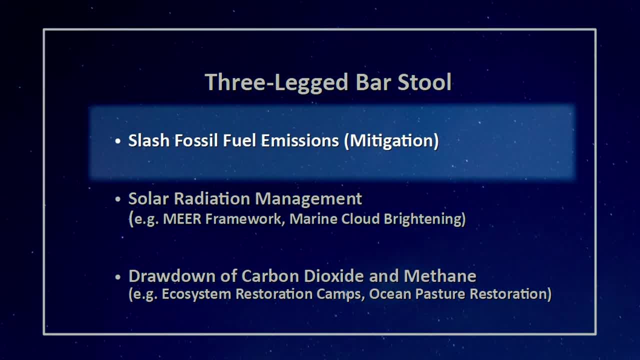 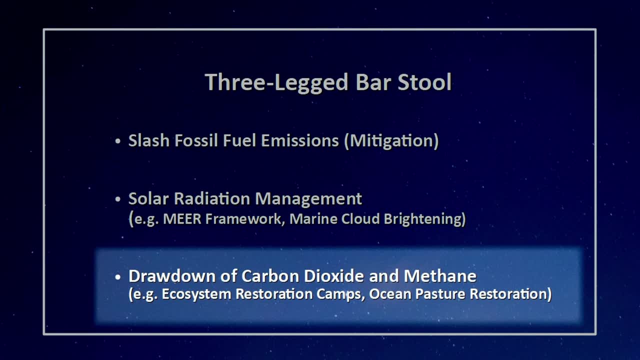 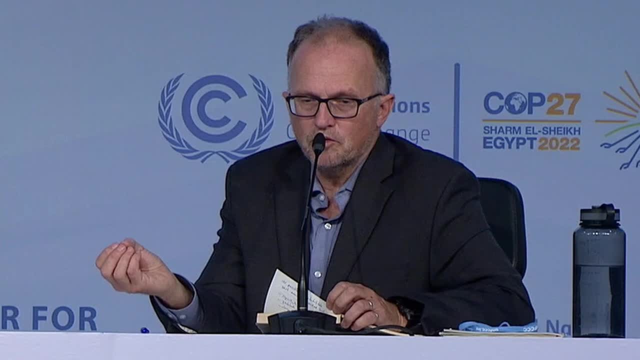 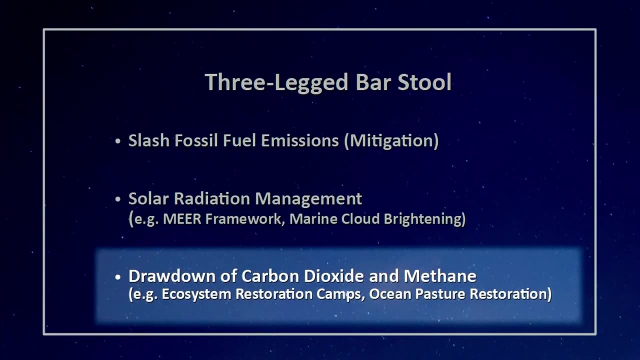 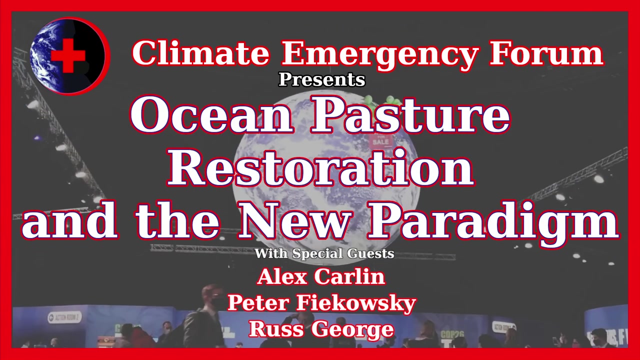 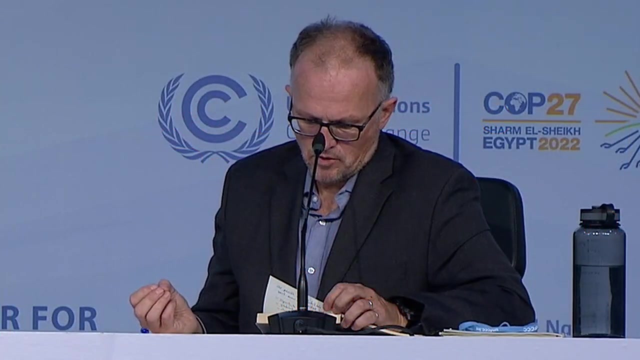 those UCI experts. I don't know if I know, if I have time, and that would be really interesting, but I don't know the reason about 돌려나 이런 것 để 다�. striving toward 소� bridge. we've never been so finished, but we still touched nails. yes, i appreciate the impact. i meanat lot of Ideas using things like a huge carbon sink, a huge way of capturing carbon. also, there's a lot of interesting work being done in the oceans. there's a lot of interesting ideas using things like ocean pasture restoration to pull carbon from the atmosphere. and the third leg of bar stool, if you like, is solar radiation management, and there are too many additional issues. but there's also lots of fascinating ideas using the first major scientific research journey that we talked about most recently, which 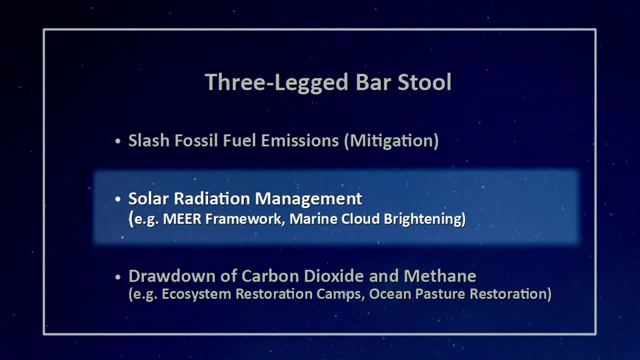 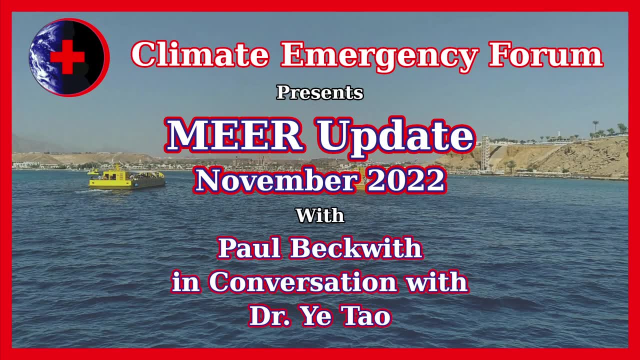 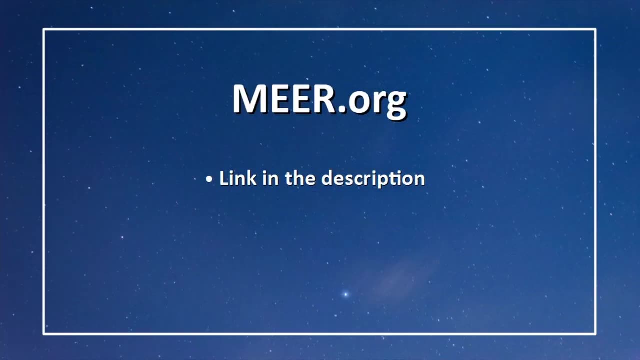 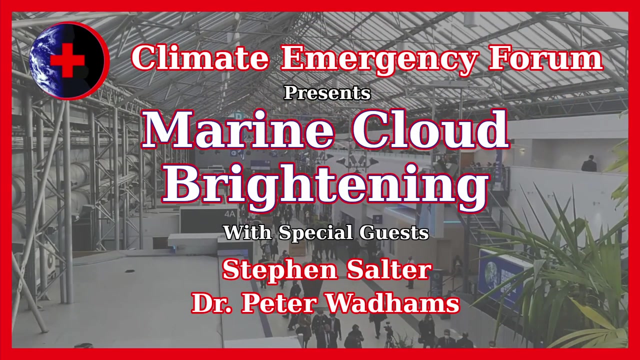 with this. I love the idea of the M-E-E-R MIR project to try to offset some of the warming, especially when we have a reduction of aerosols as we clean up fossil fuel emissions. So check out mirorg. There's also ideas of marine cloud brightening to create low-level clouds to have a 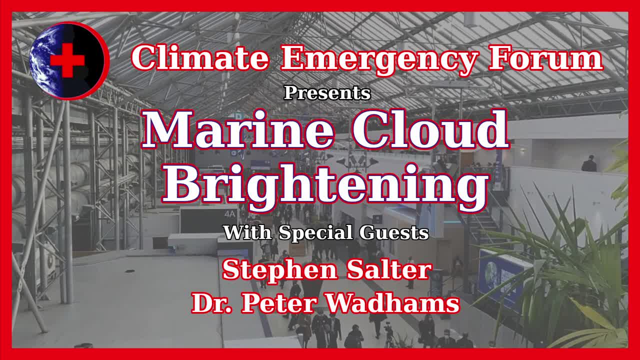 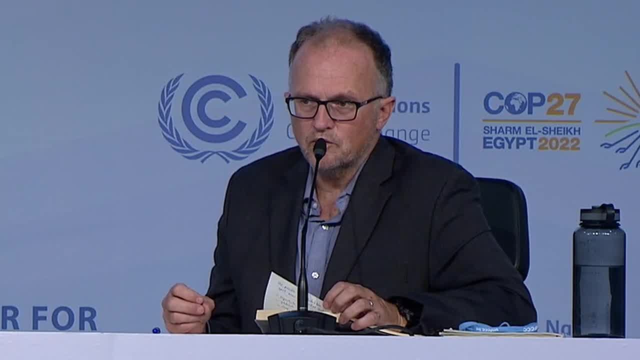 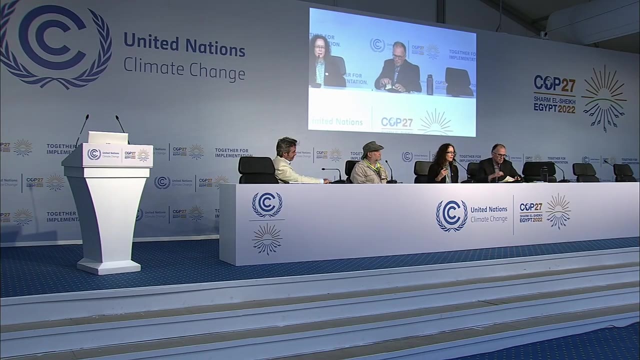 direct effect of blocking some sunlight and allowing some cooling on the planet to help get back to some sort of stability in our climate system, because we are undergoing abrupt climate change and it's accelerating rapidly to the detriment of humanity and all the animals and plants on the earth. Thank you so much, Paul. I like that you brought up a plethora of ideas and 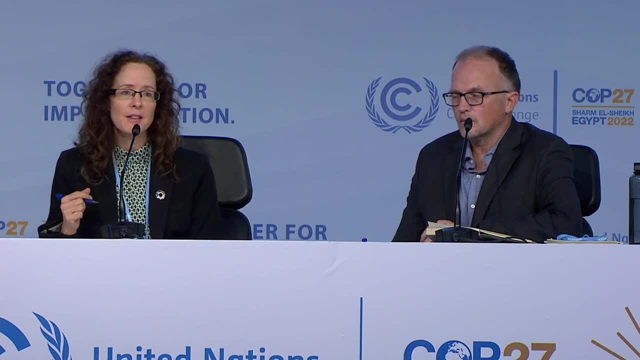 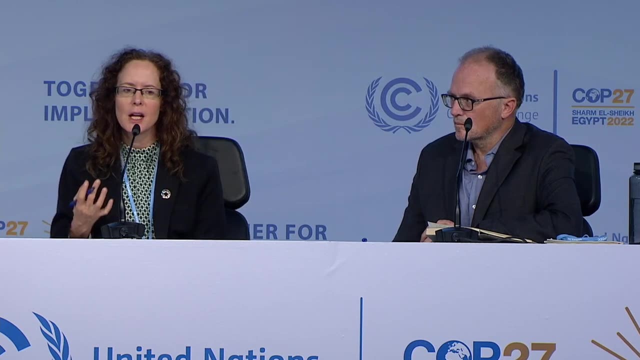 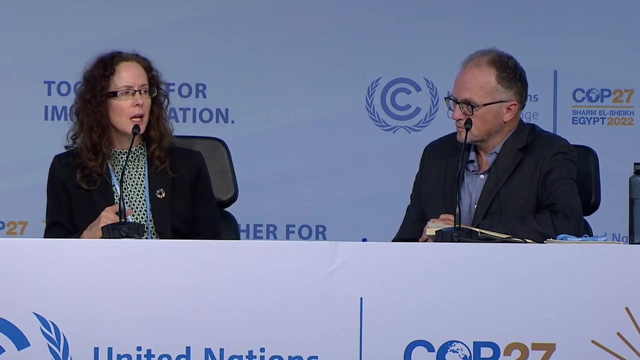 ways to restore, And I think that that is exactly what we need. We need to work with the human mind, which is so incredibly important, And when the mind is concentrated and focused, it can do so much, as you showed in that lovely, lovely video, And Paul outlined so many different ways and so many things.